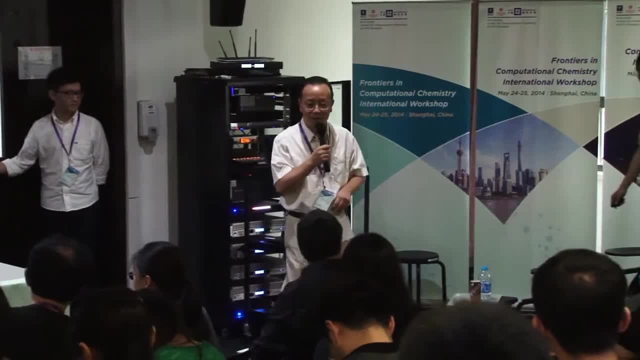 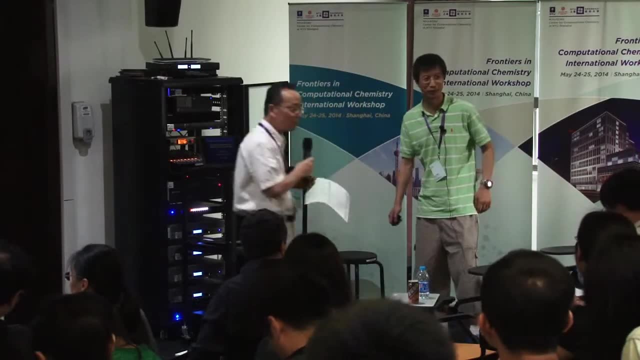 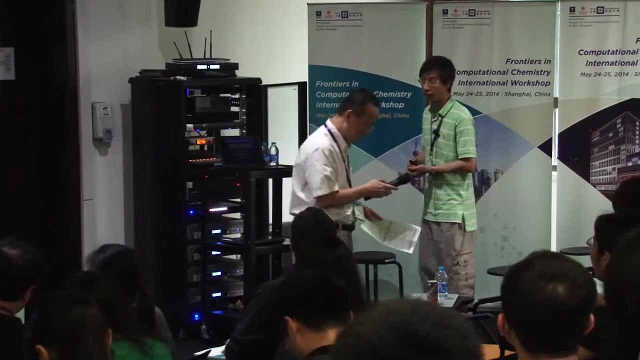 The first talk is by Professor Zhao Jiushu from Beijing Normal University. Thank you, thank you very much, Professor Zhao. Thank you, thank you very much. First, thank the organizers for this wonderful symposium And, just now, Yi Jing. you were very, very good. 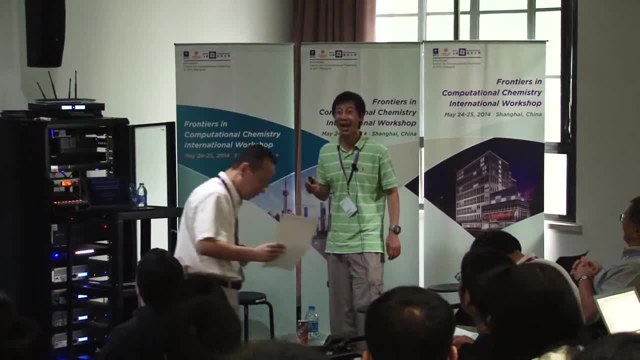 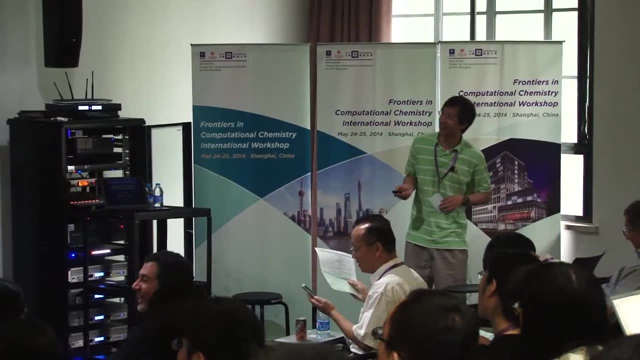 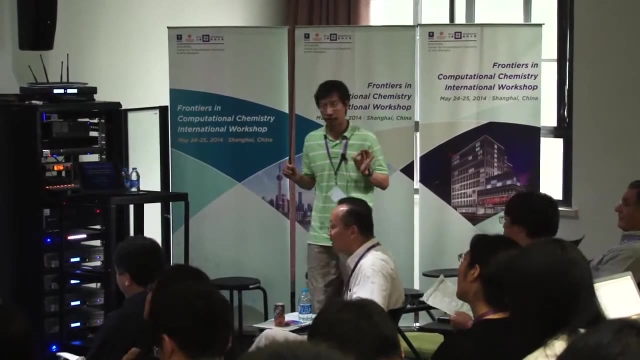 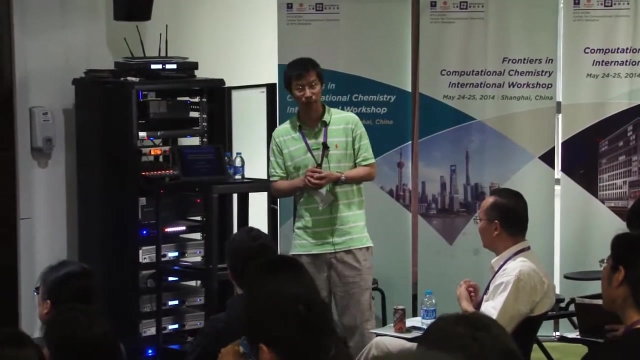 You have advanced course on quantum mechanics. Mine would be very, very elementary. I hope So. the kind of method is called quantum dynamics based on complex Brownian motion. We heard what classical Brownian motion is And it can be that quantum mechanically there is also Brownian motion. 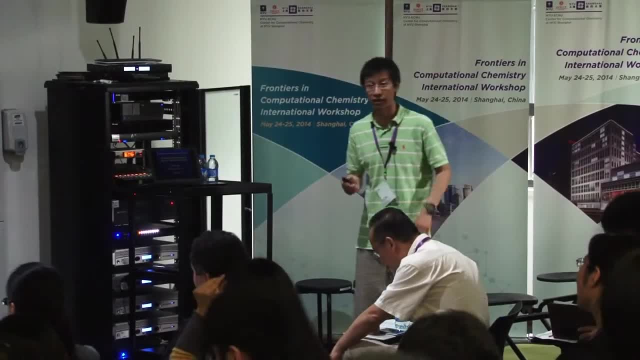 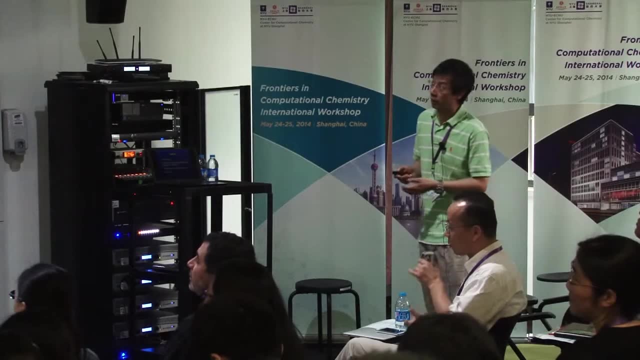 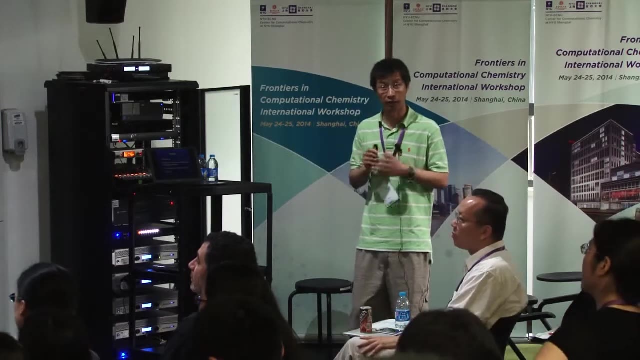 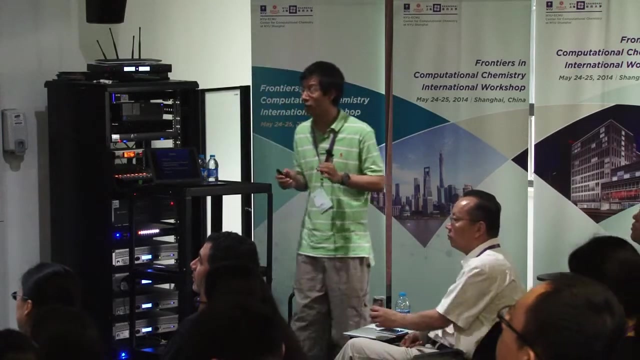 But the analysis is no longer classical, It's complex, It's not real. So the outline of my talk is the following: I will first say a few words on the motivations of our work, Then I will show you how to establish a stochastic formulation for describing the dynamics of quantum dissipative systems. 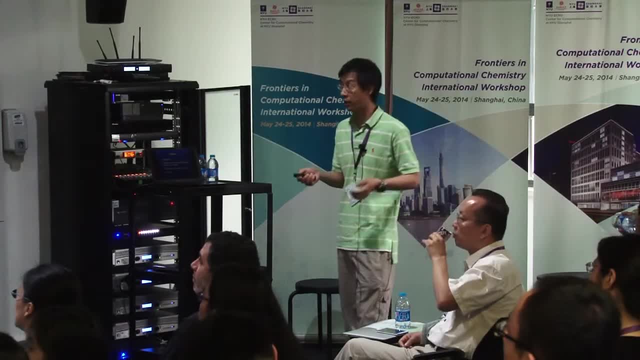 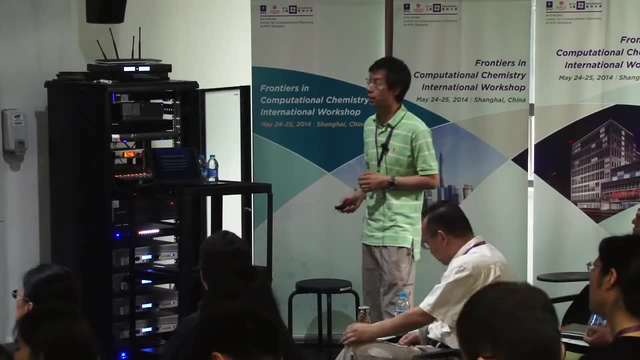 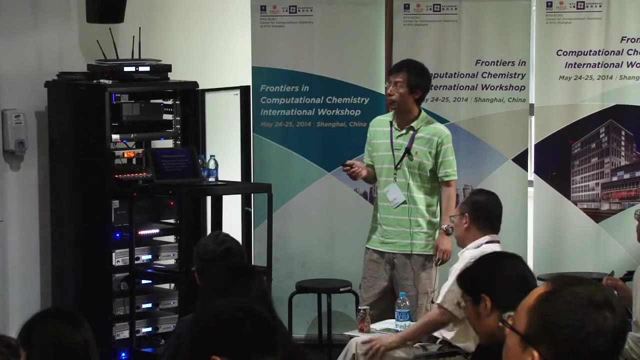 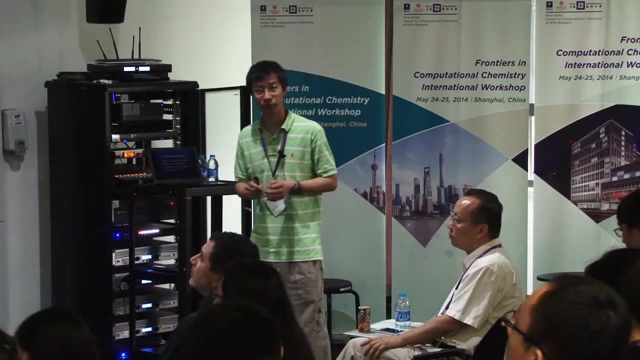 And, of course, some numerical as well as analytical analysis. The results will be shown. Finally, I will give a brief summary. Well, again, our goal is to explore dynamics in multidimensional systems When quantum effects are negligible. Well, it's really amazing that the world is quantum. 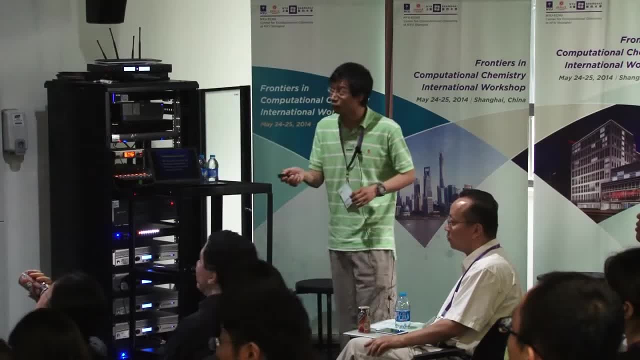 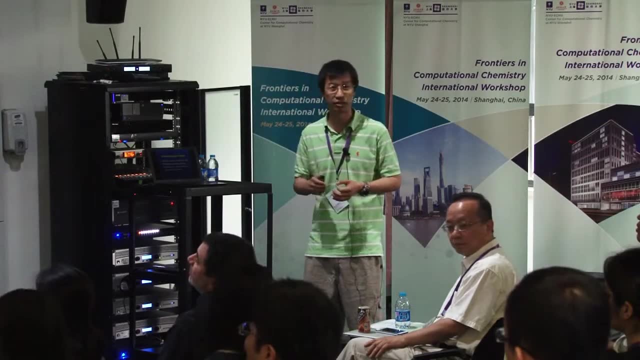 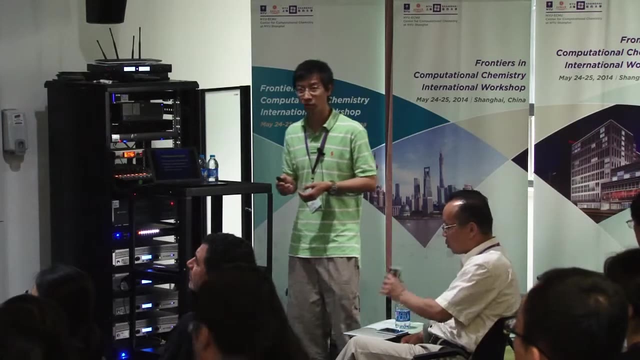 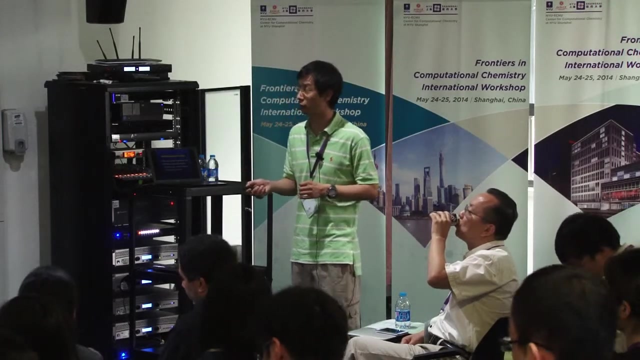 Sometimes its effects can be negligible. Then we know that we play with quantum mechanics. We know that we play with molecular dynamics. for large systems, The cost is linearly proportional to the size of the system. So how about quantum dynamics? Well, we can use different representations to study the dynamics, by either, for instance: 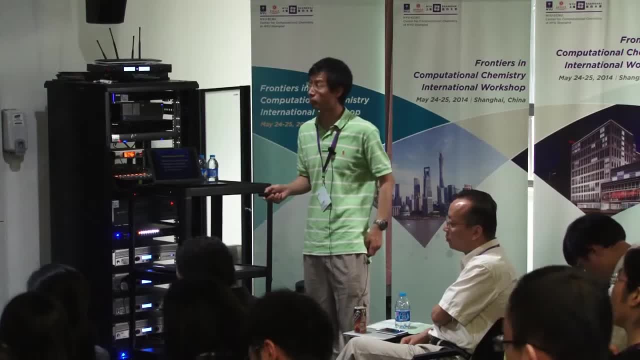 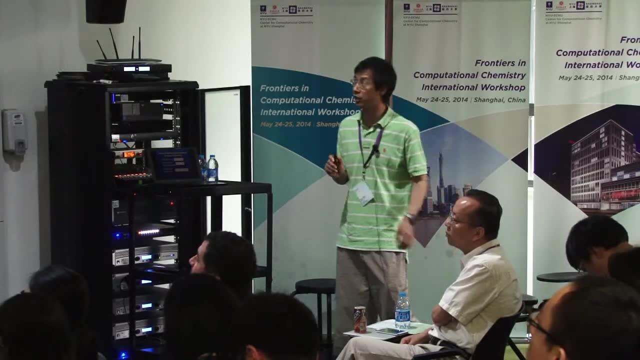 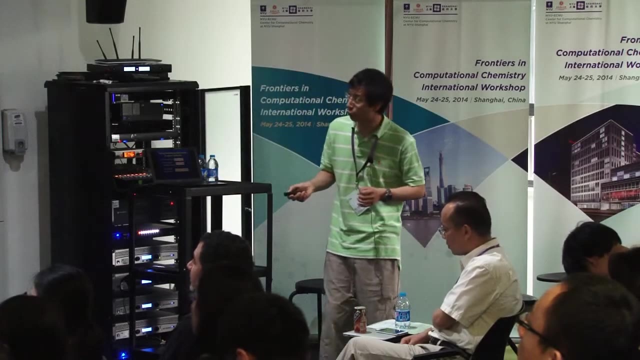 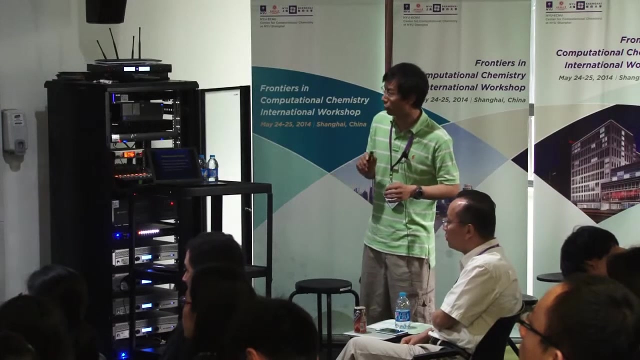 representation or possible integral. Well, we can have formal solution for these wave packets, Or we can use the integral, the plus integral, to represent our final wave packet. What's the problem? The problem is that when we use the wave packet, there's memory. 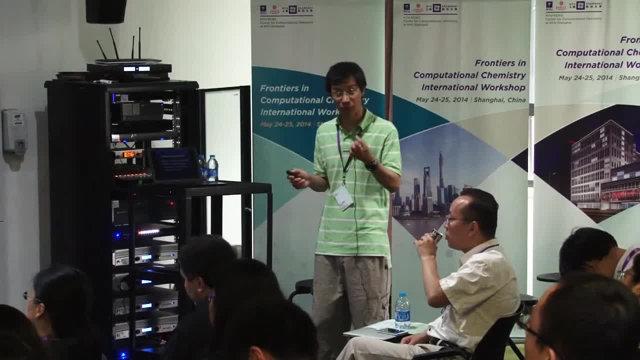 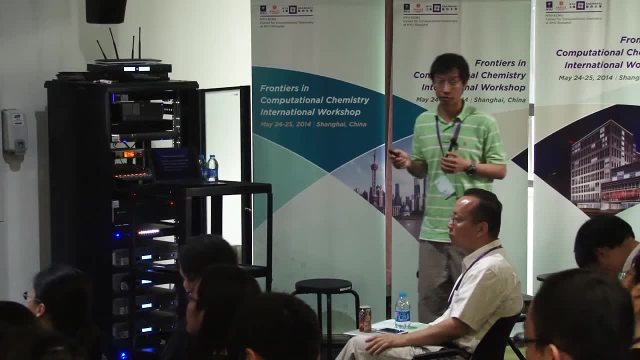 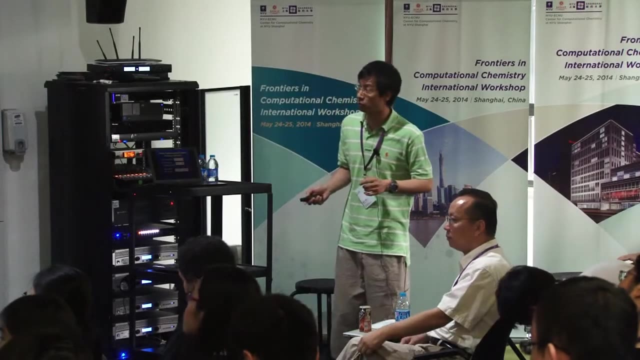 I mean the memory bottleneck. What is the memory bottleneck? The storage you require is exponentially increasing with respect to the size, And if you use plus integral, there's no size problem, But there's a size problem. So actually we will meet with the curse of dimensionality. 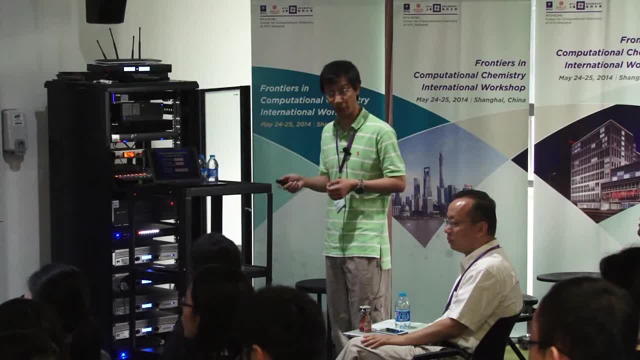 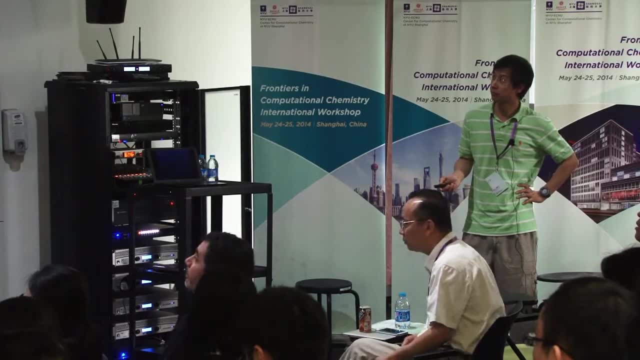 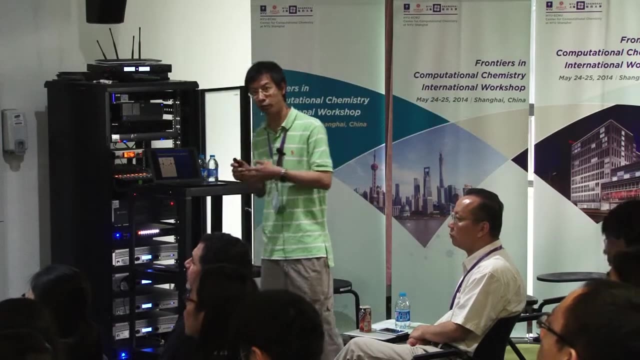 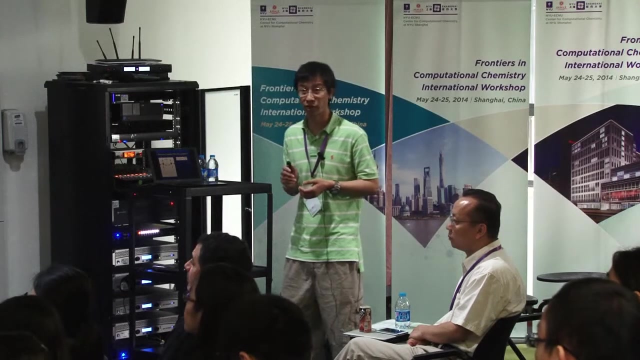 This is really a common difficulty we have to deal with in numerical calculations for complex systems. Well, Personally, a fundamental problem or interesting problem to me is the stability of Kerr molecules. Why a molecule is stable. I mean the Kerr configuration is stable. 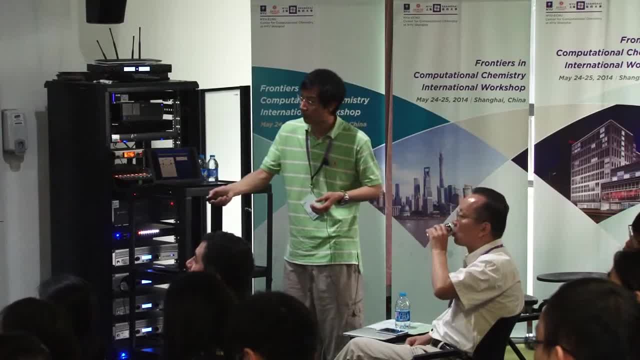 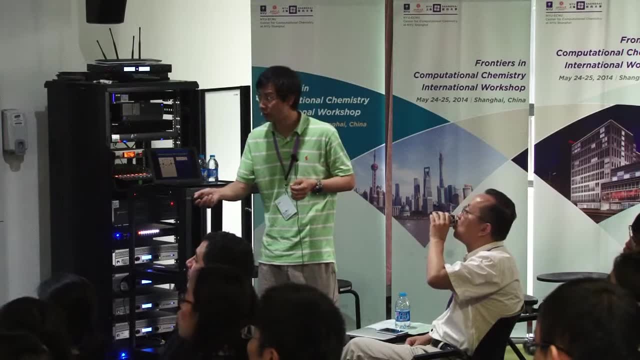 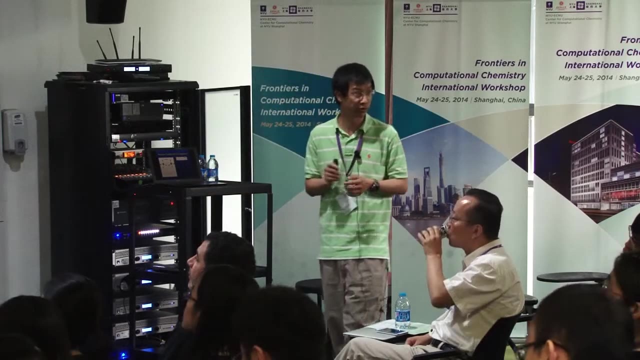 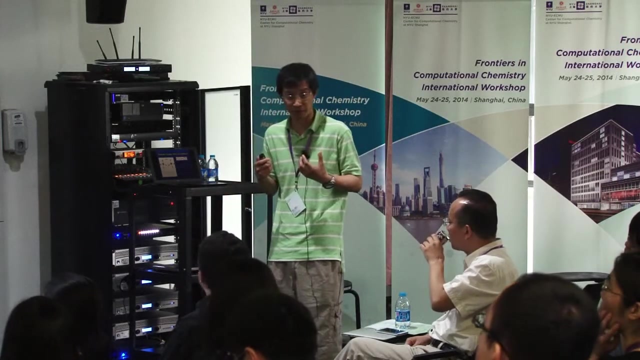 According to quantum mechanics, if you prepare a localized state, the localized state is not stationary. It should convert from this configuration to another And back and forth. This is nothing but quantum coherence. But in ordinary world, for instance, if you look at organic molecules, if you look at ourselves, 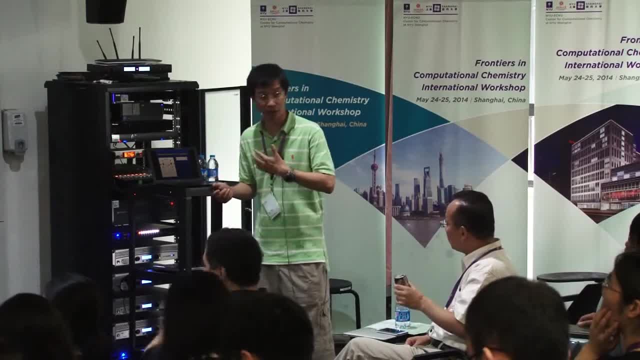 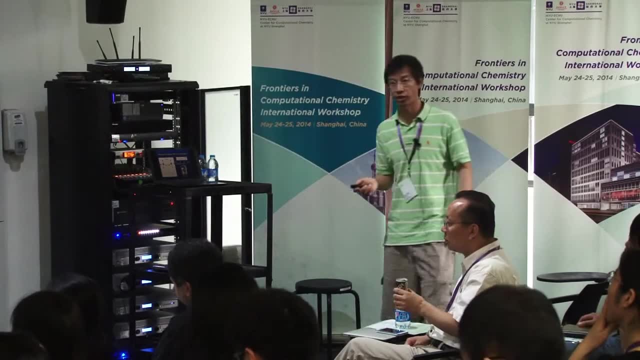 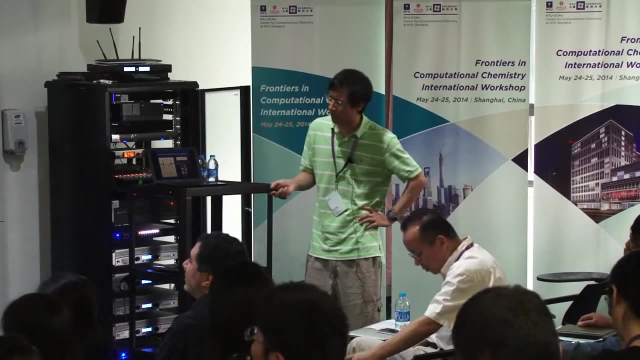 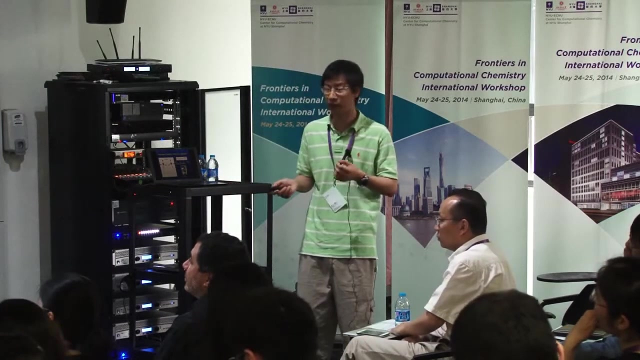 we don't change periodically from ourselves into the mirror image. Why? Why, We don't know, But this question has been raised in the inception of quantum mechanics. There won't? The very, very rudimentary understanding is that OK. in ordinary molecules, the barrier is so high that whenever you prepare a localized state, it will be there. 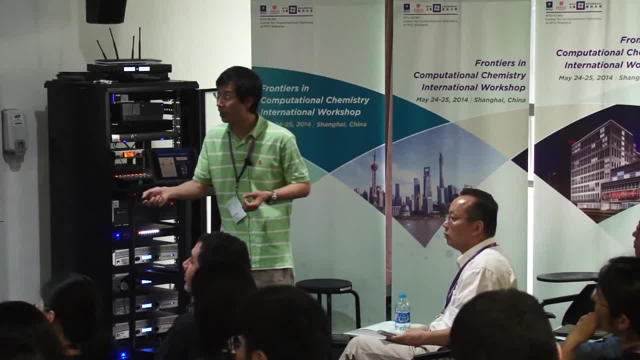 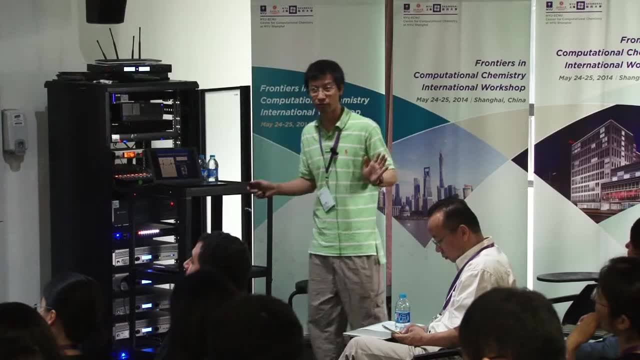 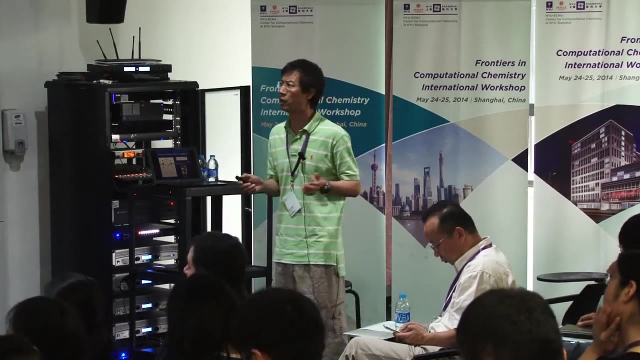 So it is stable. But it doesn't answer the question why the nature wouldn't let the molecule be in this stationary state, the lowest energy state. So well, currently we understand this. OK, the molecules are known. They are not isolated. 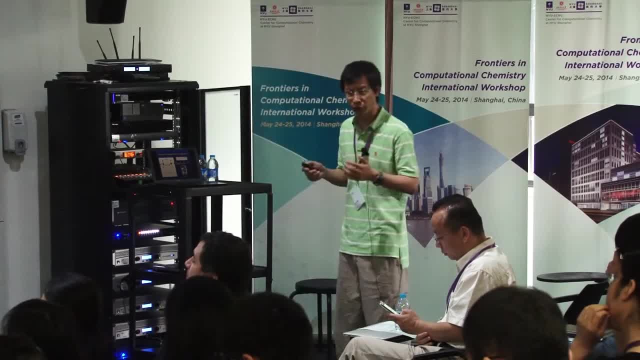 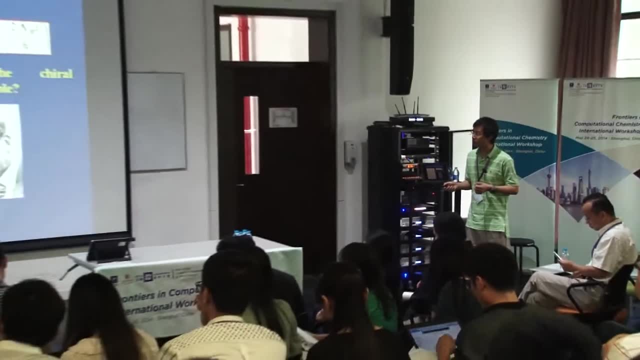 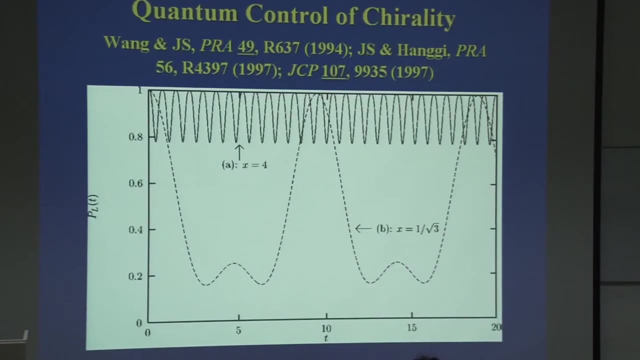 They are coupled to the environment. When we know the coupling, the coupling effect, then we may know the intrinsic mechanism of the stability of Kerr molecules. This is really what we want to explore. OK, we have done something on the quantum control a couple of years ago. 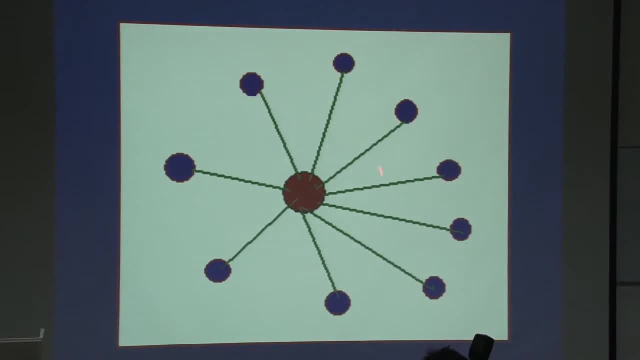 I didn't escape this. Now the question is that we want to understand And the dynamics of subsystem, here labeled by right. Why, Because of the interaction, the dynamics should be modified, sometimes grammatically. How can we deal with it? 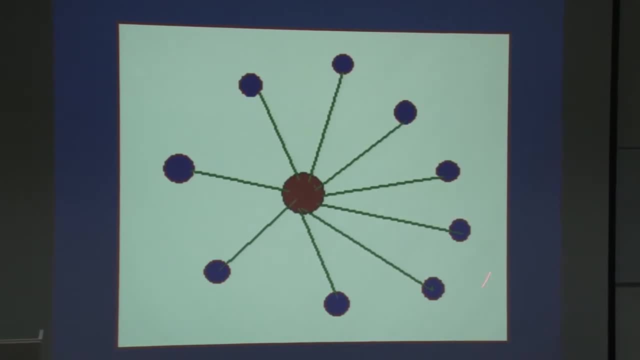 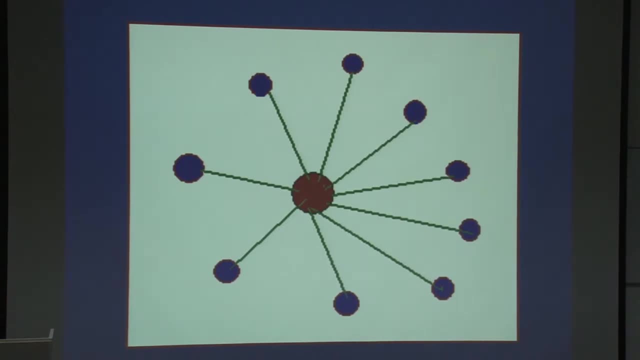 Again, let me pose a question. We have a whole system, system plus the bus. We are interested only in the physical properties of the subsystem, here labeled in red. But because of the interaction we know the dynamics of other properties will change. 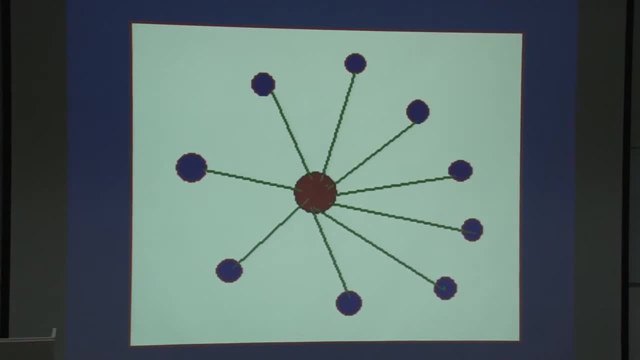 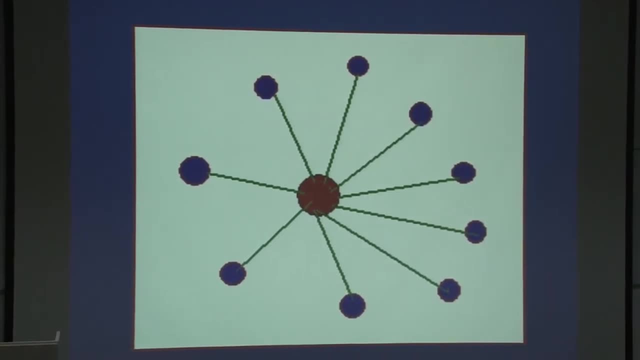 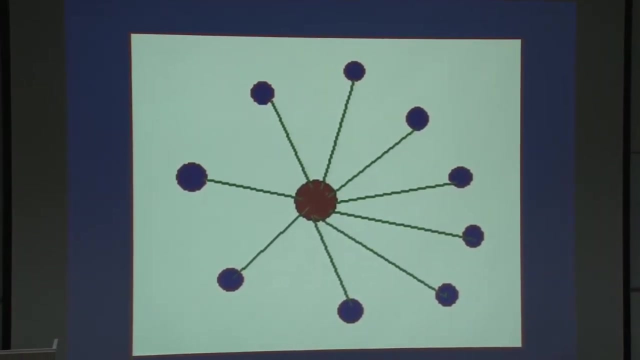 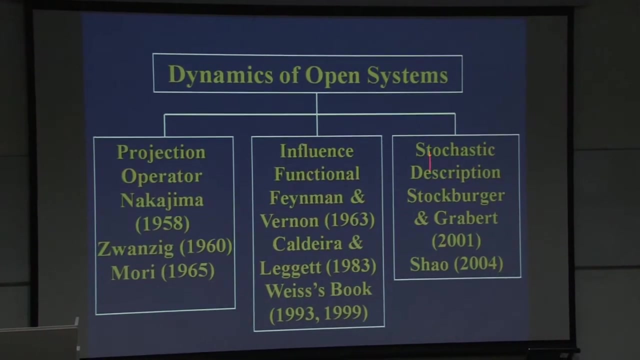 But how? Now let's suppose we know the dynamic behavior of this isolated guy and the isolated environment. Then can we know the properties of the system. Of course there is no interaction. The properties will not be modified anymore. So we have to do the introduction to the histories. 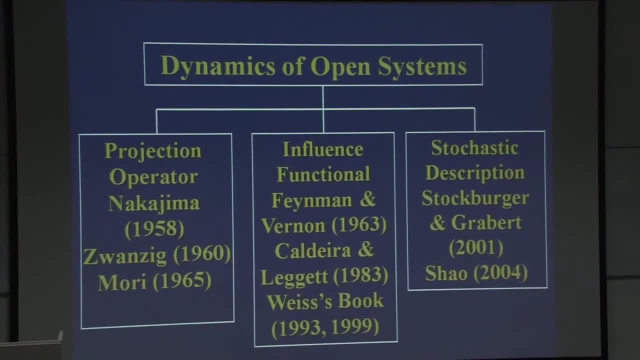 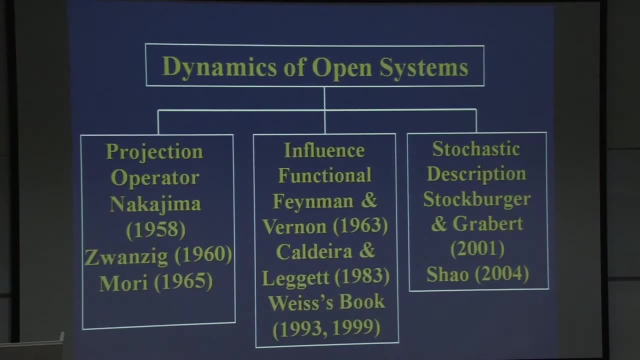 Many years ago. when the interaction is weak, one can use a production operator to do perturbation, And this technique has already been widely used in spectroscopy. A couple of years later, Feynman and Vernon developed the influence function now and popularized by Caldera and Leavitt. 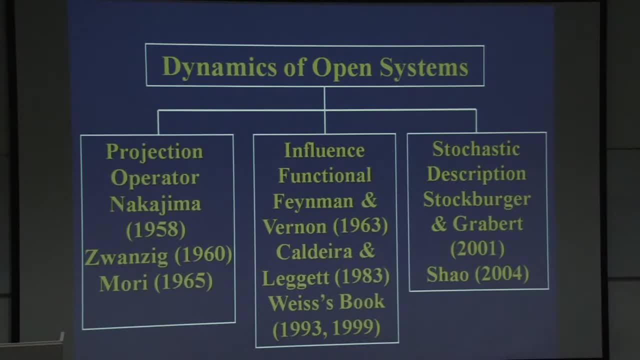 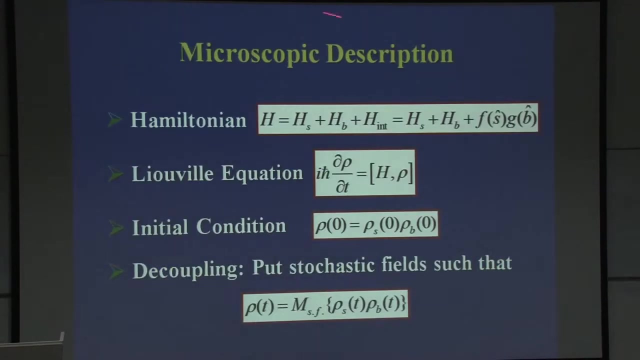 And today I focus on different methods, including the description developed by Stockburger and Grebert. We further developed, Of course, the phenomenological idea was initiated by Kuhl a couple of years ago. We now look at the spectroscopic description. 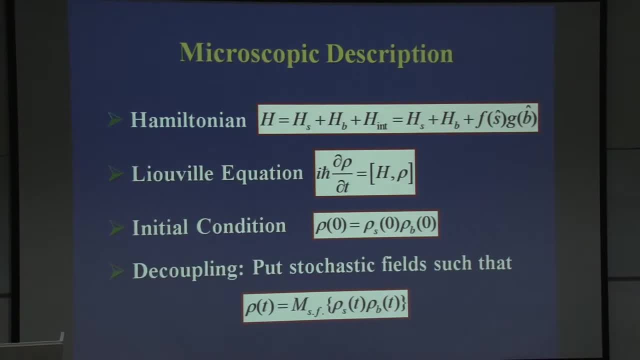 So we think about the open system can be described as closed system. It consists only two parts or subsystems. One is the system, Another is the bus. of course, If there were no interaction, we know the system and the bus will evolve independently. 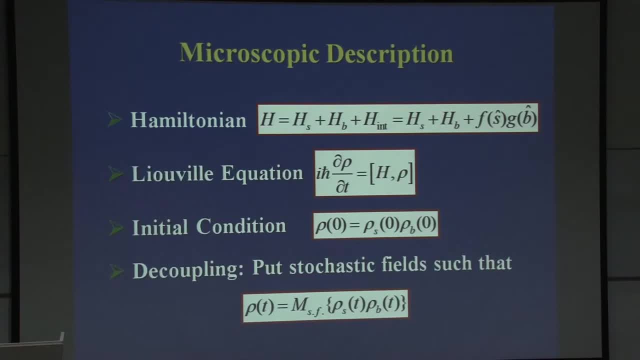 But the beast is the interaction. Again, let's assume we can solve the dynamics of the system and the bus separately. Now the question is that how can we deal with this interaction? This is a force or field or a product, This is a form, whatever you call it. 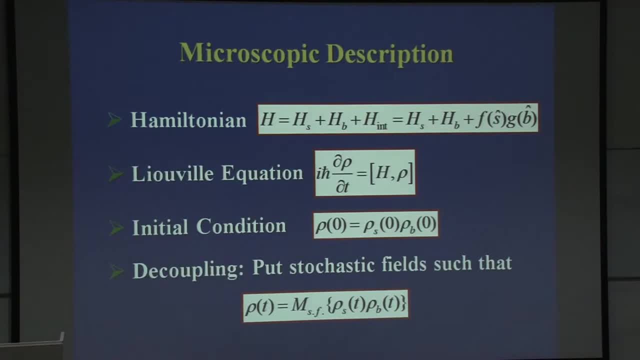 Now we look at the dictating equation of motion, the neural equation, Given an initial condition- again, if we can somehow to have this form. I will explain a little bit. the system and bus evolve independently And by combining them. 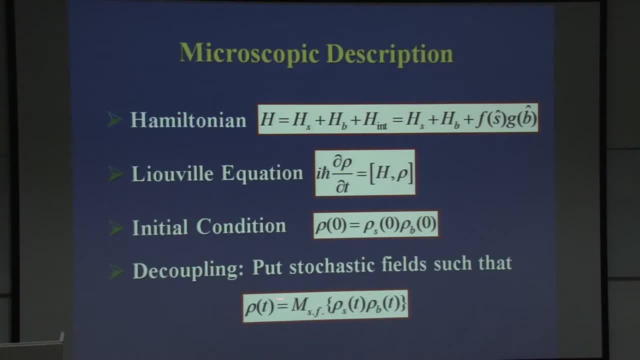 we do some further manipulation so that we have the dynamics of the whole system. What does it mean? It means that we have to deal with this interaction so that part of the interaction goes to the system, the other part goes to the bus, so that somehow we have independent or non-interacting system on the bus. 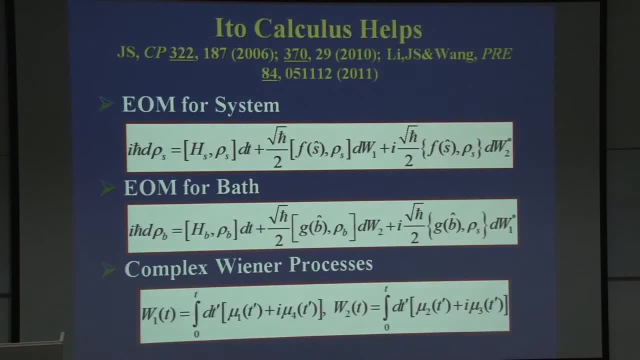 Then we can deal with them independently. Well, it can be done. It's very simple. If you are familiar with Ito calculus, then you can write down two equations for motion. One is for the system, the other is for the bus. 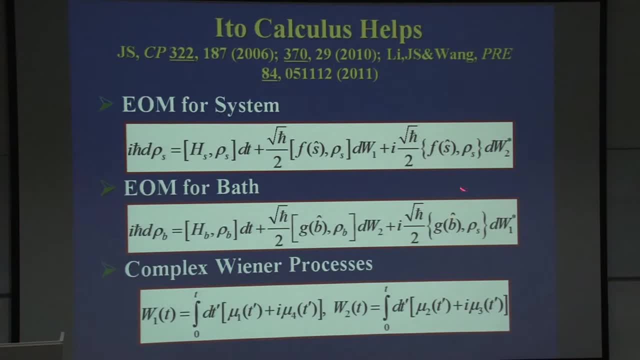 Well, the price we paid here is to introduce the complex noise, web noise, And you can show that if you do the stochastic average of the combining motion. by combining I mean we think of the product, of the density matrices of the system and bus. 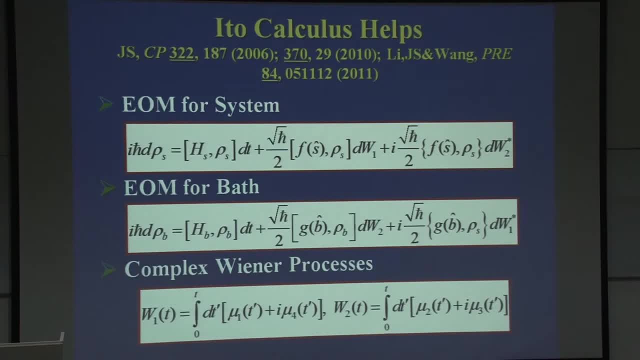 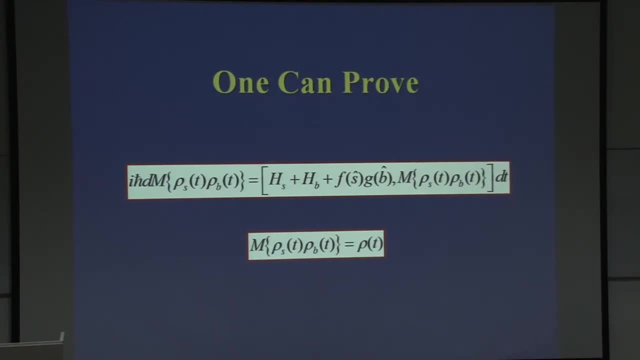 and you try to derive the equation of motion, you will find that it's nothing but the original Buber equation. That means we proved that the independent motion of the system and bus give the exact dynamics of the whole system. It's very simple. 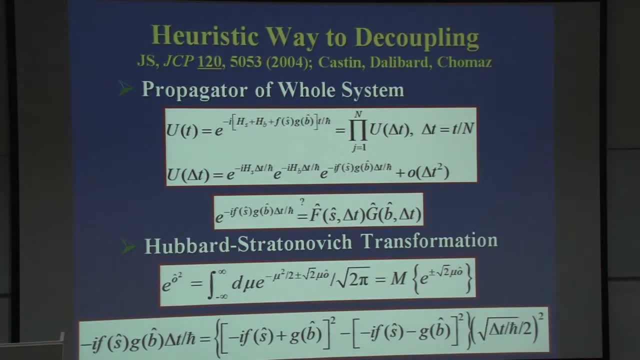 Well, maybe if you are not familiar with Ito calculus, it's not very easy to follow. I will give you a heuristic way to decouple the system and bus. This is also a original derivation we developed. Now the dynamics is fully determined. 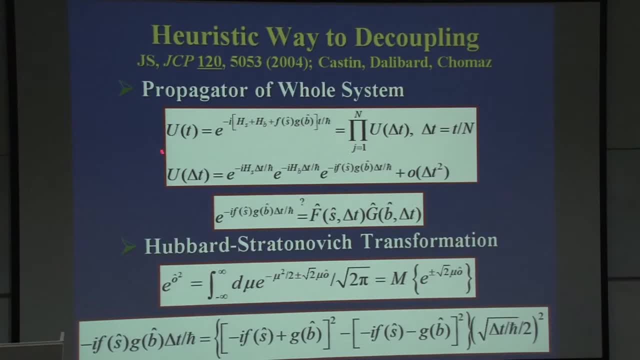 by the propagator of the whole system For a short time step. the propagator consists of three factors: one due to the system, the one due to the bus, Of course. the other is due to the interaction between the system and the bus. 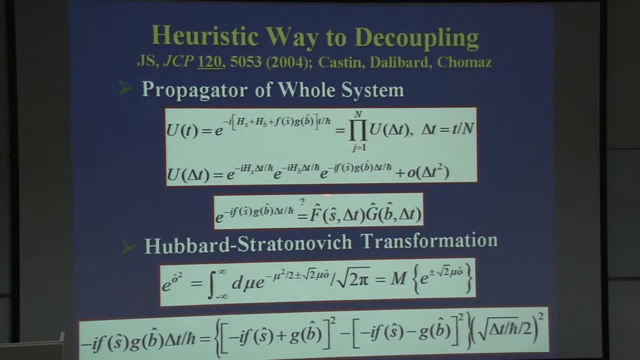 Now again, if we know how to group these factors into two subgroups or into two factors- one goes to the system, the other to the bus- then we have independent propagators. Quite a simple idea. How can we do that? 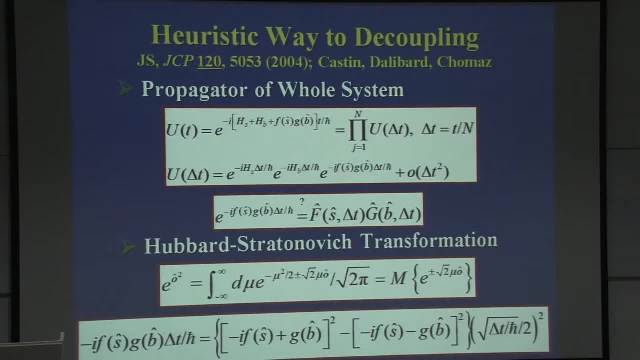 Okay, because we suppose the interaction is product form or false. field form is not specific, It's general. And for general interaction you always allow to write it into some of the product forms. Then we use a Gaussian integral Or in physical terminology, 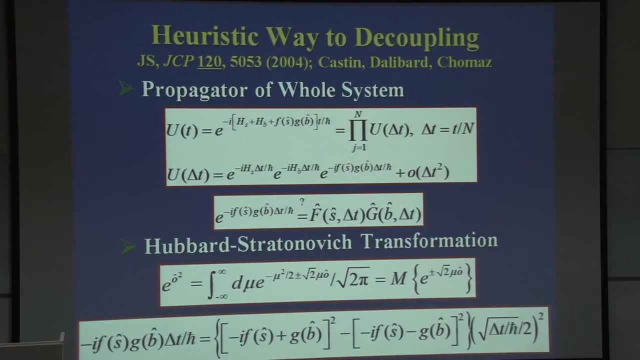 it is Albert's spectrometry transformation Here for any operator. d squared means that there is self-interaction. When we do the integral it means that there's no interaction at all, But it interacts with scalar field. So we introduce a mu. 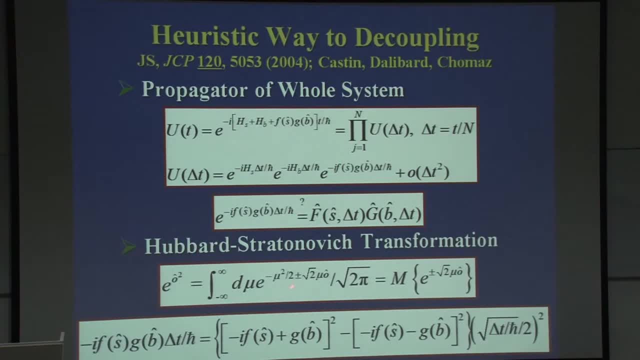 Now, if you reinterpret this Gaussian as probability density, then you are allowed to write this integral as a stochastic average or random average of this physical quantity. It's very simple: There's no longer self-interaction, but the system is interacting. 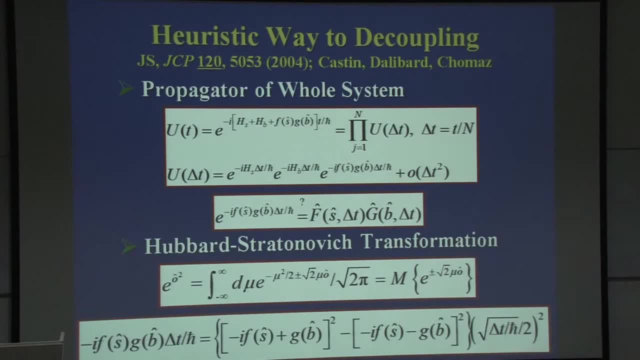 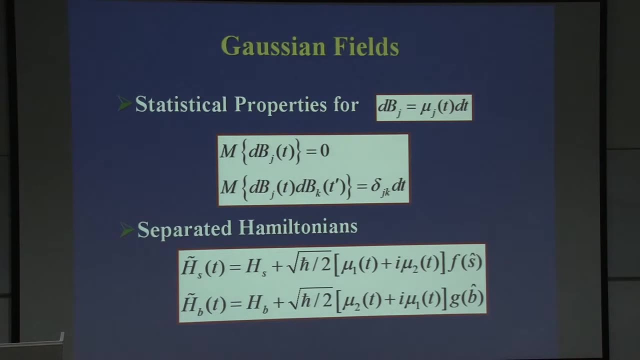 with the field produced. So for every time step we do the same thing. It means that you have a bunch of random numbers And it's nothing but the Gaussian process. It's like noise, So you can prove rigorously. 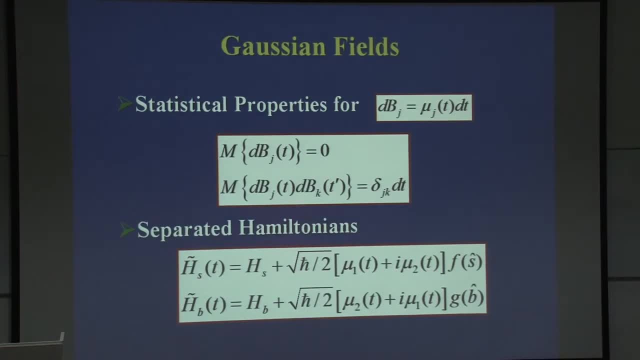 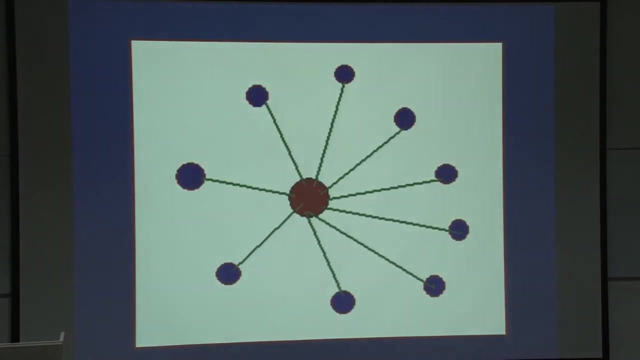 So we have independent system and independent class. Now, by independent I mean there's no direct or quantum interaction. They are correlated Because they are subjected to the same complex noises. So I would like to use this picture to illustrate what we have done. 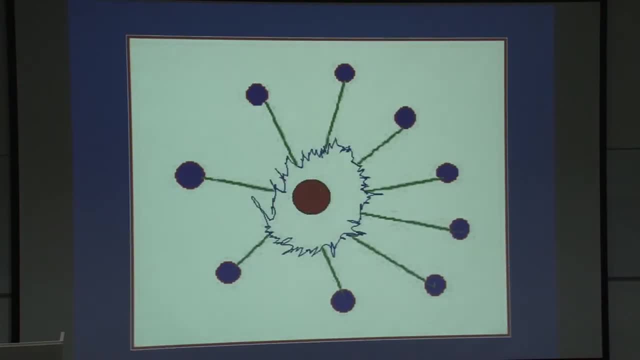 Originally we have interaction. We have a system of bars. By the mathematical manipulation that is, we introduce the stochastic field. There's no longer the direct interaction between the system and the bars, but they are correlated because they are moving with the stochastic field. 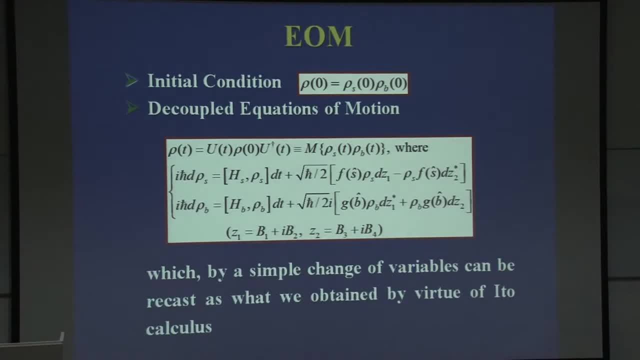 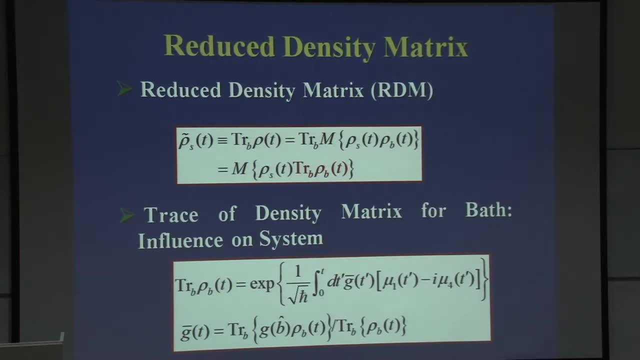 So, so far, so good. We have the spatial motion, blah, blah, blah, not to get into details. And okay, here is the key point: We don't want to know the exact dynamics of the whole system, because the information is too much. 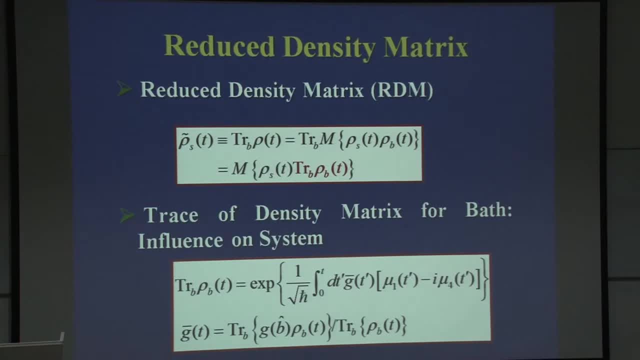 What we want to know is the dynamics associated with the system. So reduce the density matrix is sufficient. So we know that the exact dynamics or the exact density matrix can be written as the combined system of the bars one. Of course we do the 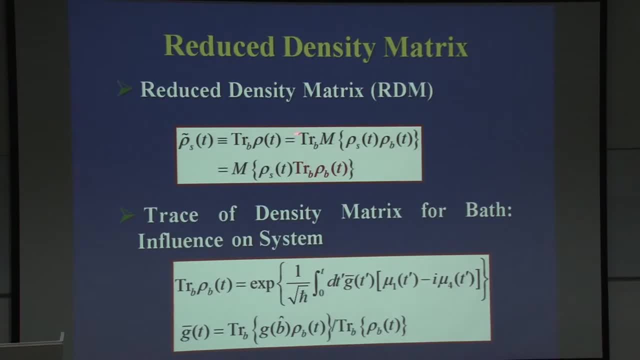 stochastic average. Let's change the order of the creasing and the stochastic averaging, Then we have a simpler form. Look, this is the twist of the bars with the density matrix. At the very beginning it is one, Now again. 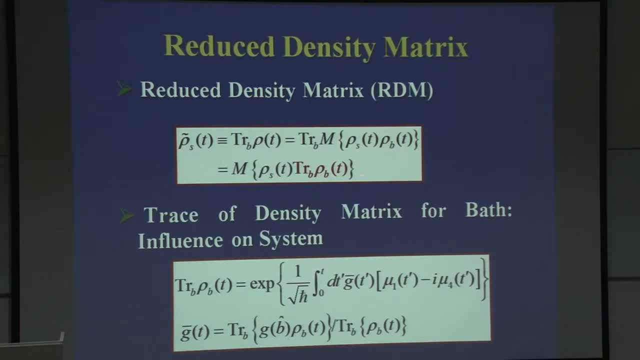 because of the complex noises, the Hamiltonian is no longer formation, So the twist will not be preserved. It's not adapted at all. So finally, we can write down this twist of the density matrix from the bars in an integral form. 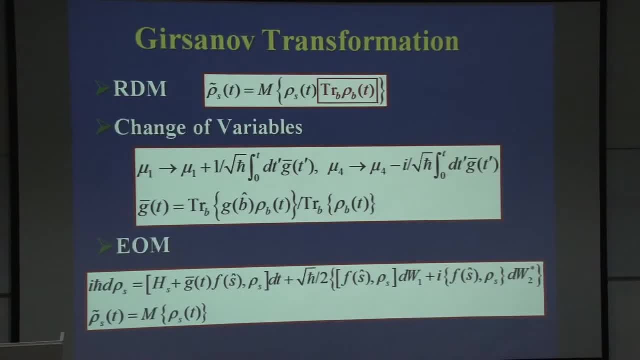 Then we do some change of variables. It's very simple, Although mathematically it's called transformation. It means that we absorb the influence of the bars into the probability density of the original red noise. Then we have an equation of motion for the system. 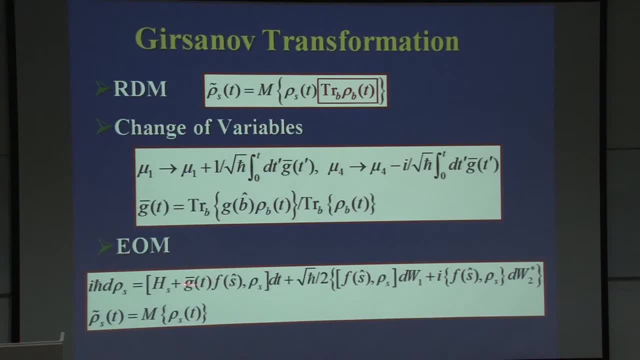 Now, when we are able to do the stochastic average for the random system, we will have the exact reduced density matrix. So you may ask: what is the influence of the bars? Of course there is Here- we call it- bars-induced affinity. 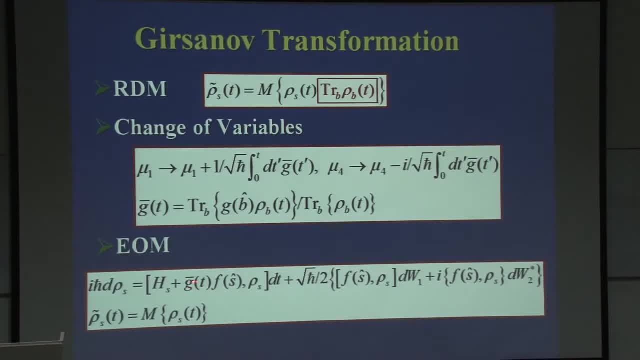 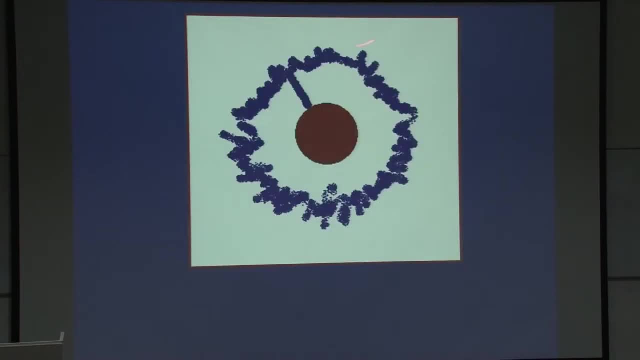 All of the impact of bars is reflected in this property, scalar one. Of course, it's complex Again, I would like to use this picture to illustrate what we have done. So we convert the influence of the bars into a complex, stochastic field. 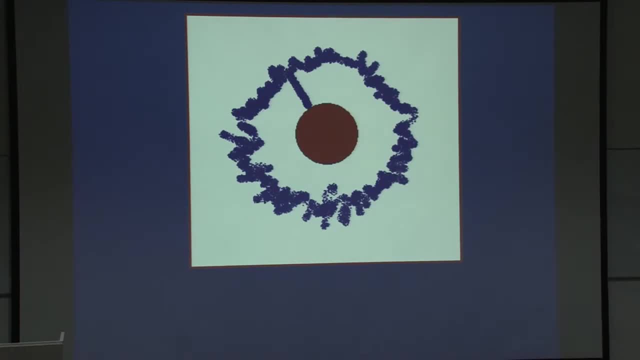 so that the dynamics of the system is subject to the stochastic field. It is rigorously a mathematical formulation. So whenever we can calculate this stochastic differential equation and able to do the stochastic averaging, everything is fine. So the problem is that 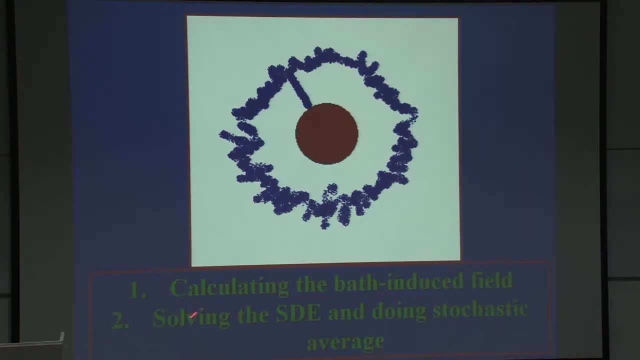 OK, how do you calculate the bars-induced affinity? The second one is: how do you solve the stochastic differential equation and do the stochastic average? If these two questions can be answered, perfect free lunch. Because again, we have already reduced. 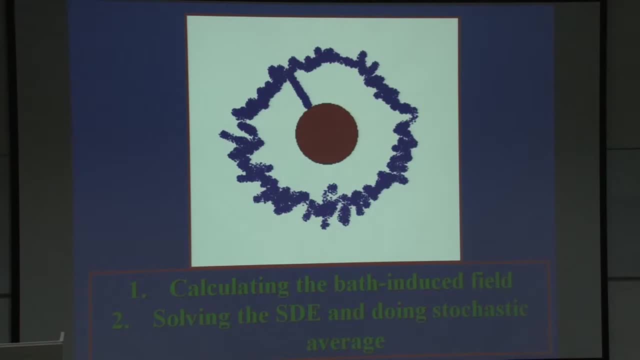 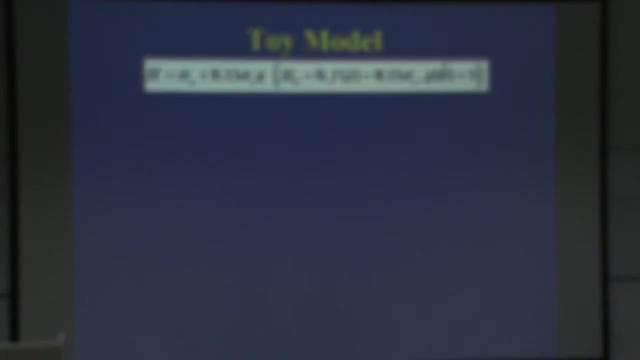 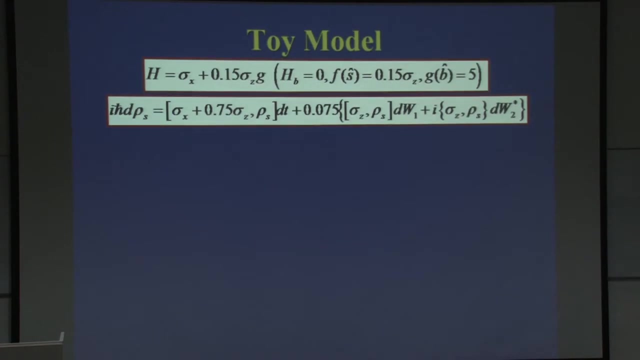 the number of dimensions. Now let's look at the towing model. Let's play with it to see if the idea works. It's a two-level system in a static field. Let's interpret this static field as a field, as the bus. 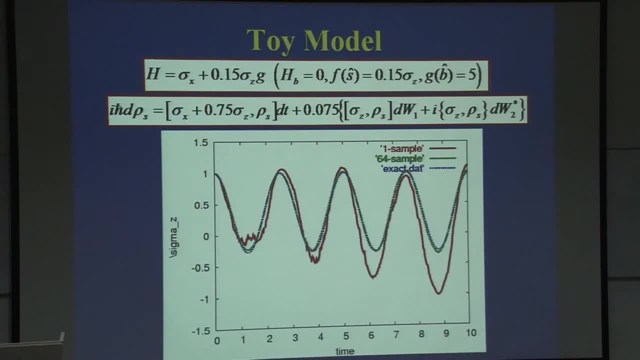 Then you can write a few lines of cues to do simulations. It's quite simple. So the blue dots are the exact solution because two by two matrix, you can diagonalize it. you know the exact dynamics If you use one sample. 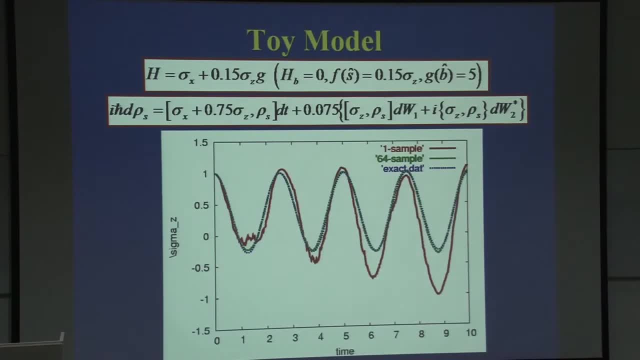 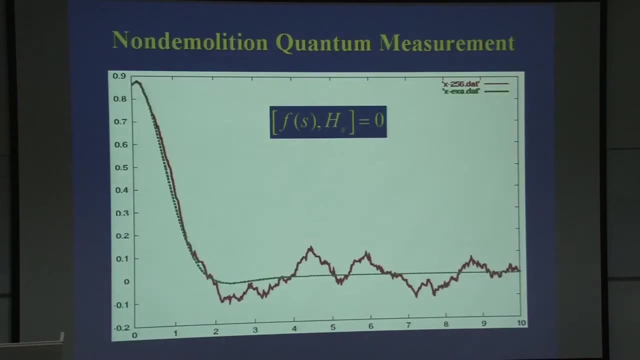 your libation here, the red line. the result is poor, But you can easily increase the number of somethings up to 64.. It almost reproduces the exact data. So the single idea, it does work And we also play. 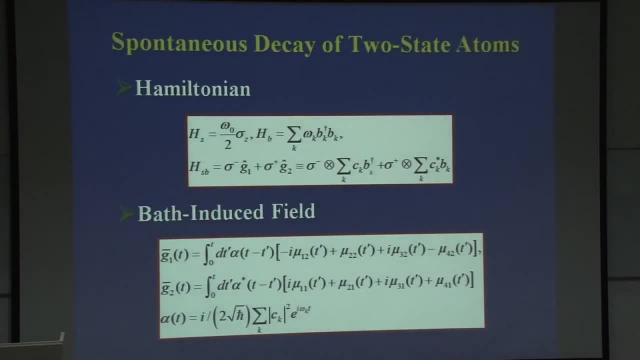 with other models and we skip this one. But let's look at a more realistic problem: a spontaneous state of two-state atoms. Here you have a two-level system. again, you prepare it in the excited state Because of the vacuum. 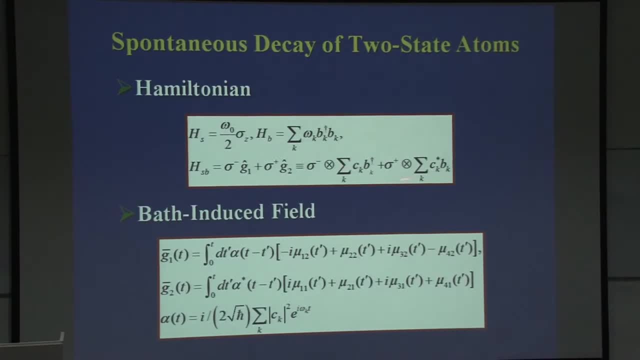 the system will decay to the grand state. Now there are two interaction terms. Again, as I've explained, we can deal with this kind of interactions or the sum of them. The price is that we have to introduce a pair of stochastic fields. 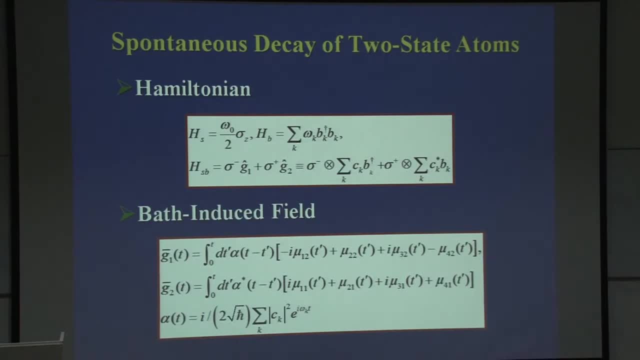 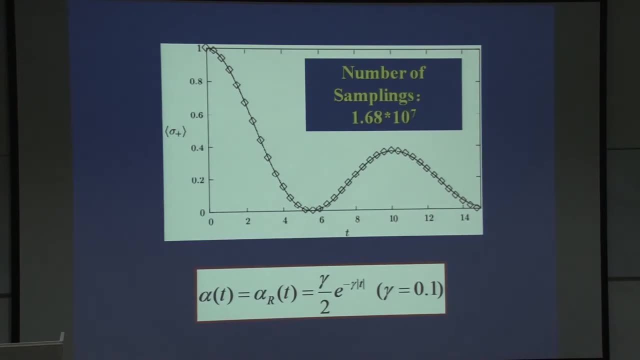 So this is linear system. You can easily write down the bus-induced field, blah, blah, blah. Again. you can write a few lines of cubes to do simulations. The results are very good. So the straight line is the exact result. 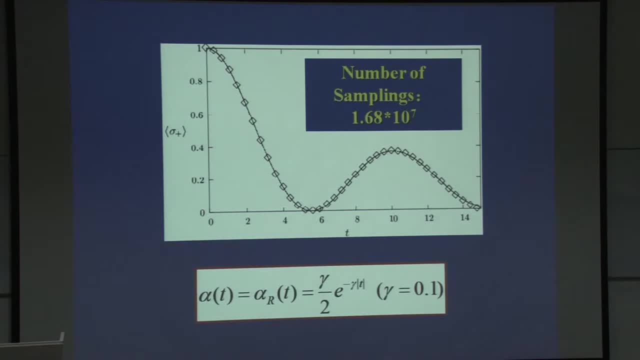 because this model, precisely, is the exact mass equation. You can solve it numerically, you can have dynamics. The diamond represents our simulation, with that Almost perfect agreement. well, well is perfect for this time range. The statistical errors go very fast beyond that. 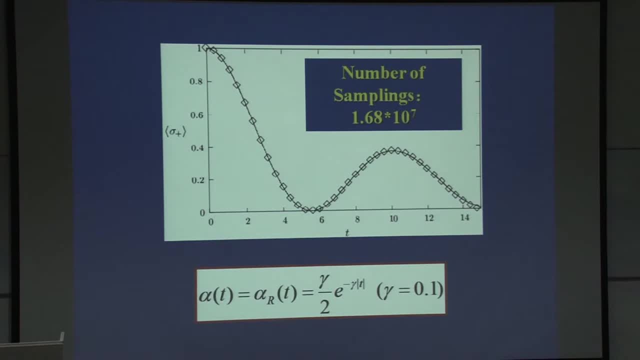 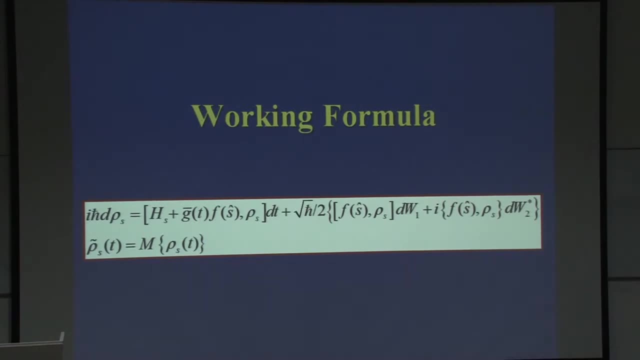 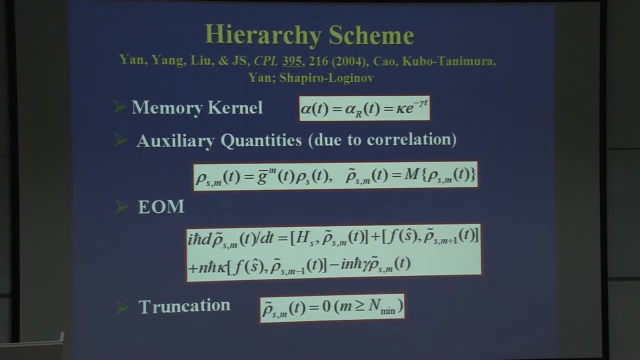 So it seems that the plain implementation does not work for longer times. So then we have to think about other way to do it efficiently. This is why we developed the hierarchical equation, the hierarchical equation of motion methods. Now let's suppose 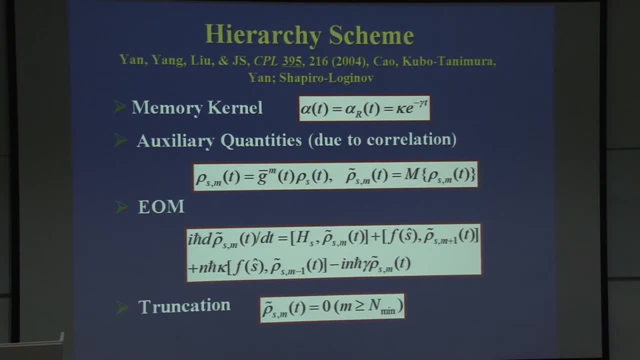 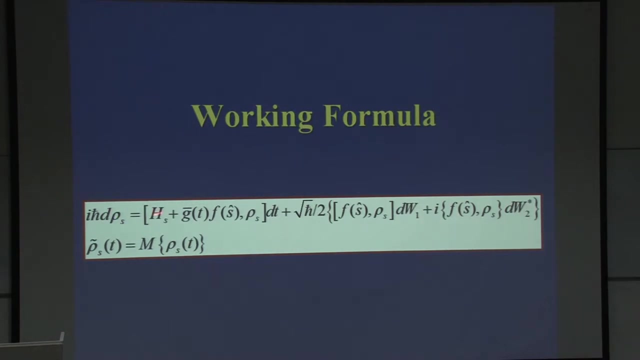 the response function or the memory function for this bus-induced field has exponential form. It is nothing but the Ohmstein-Wuhlenbeck noise. Then you do the. this is working formula. We do the average. we do the average. 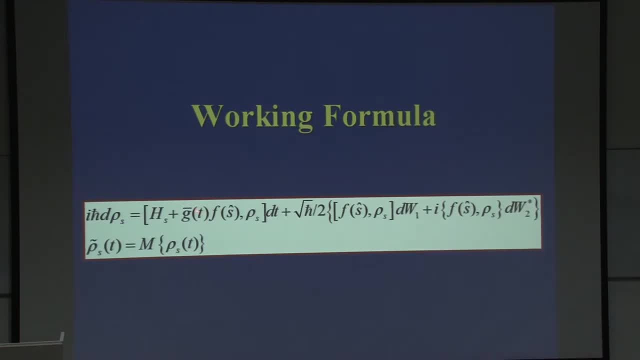 we do the average on both sides, We find that, okay, this is a complex, this is a complex stochastic noise. There is correlation between this and the stochastic density matrix. The average of the products is not the product of the average. That's the problem. 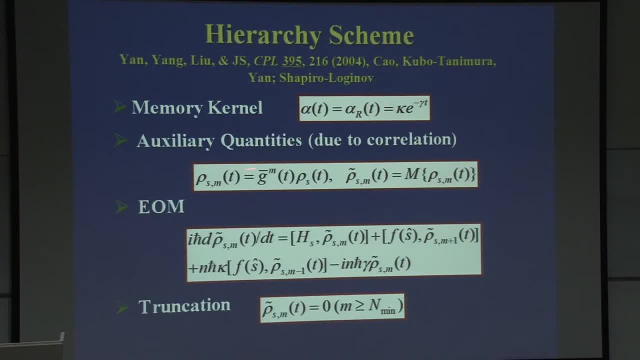 that's correlation. So again we have to introduce some of the zero rate quantities we defined in our paper. So Yijing has talked about the physical menus At the very beginning. we know that it's nothing but the hair order correlation. 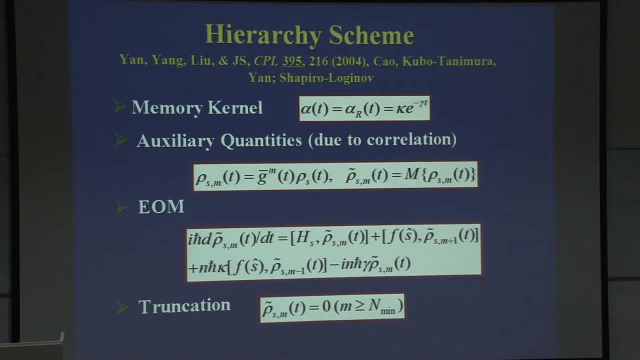 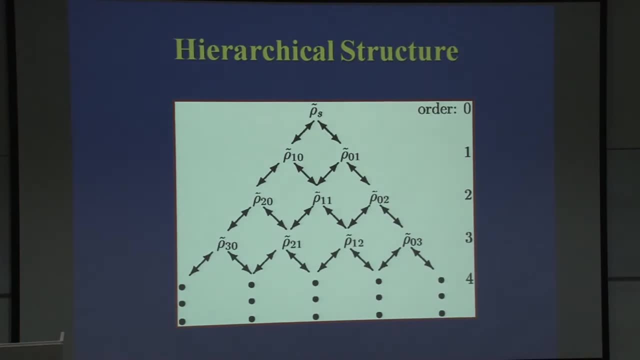 of bus-induced field with the system, So so on and so forth. We use this picture in our original paper to illustrate what the hierarchical equation motion method means. okay, This is the guy. we want to calculate the redundant matrix. They are of zero rate quantities. 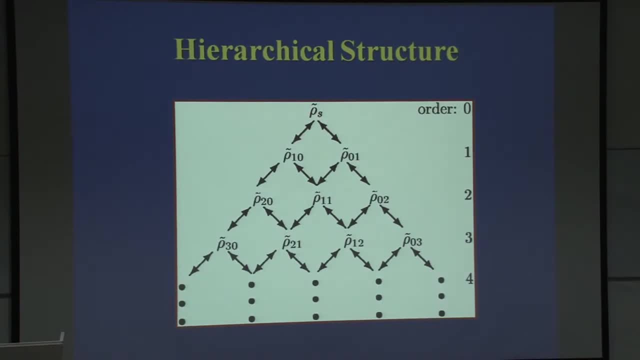 because they are related with each other and layer by layer. We know that the interdependence between this layer and that layer reflects the hair order correlation of the noise. So the interdependence becomes weaker and weaker. To some point we can make a truncation. 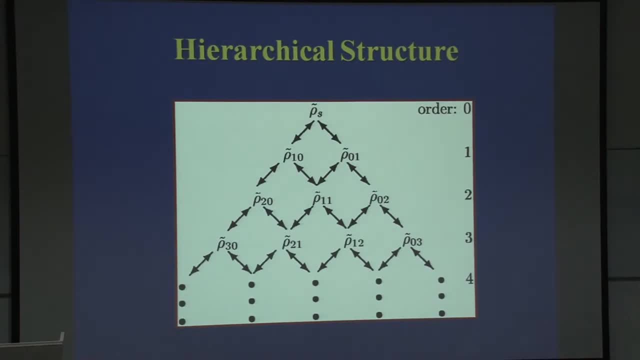 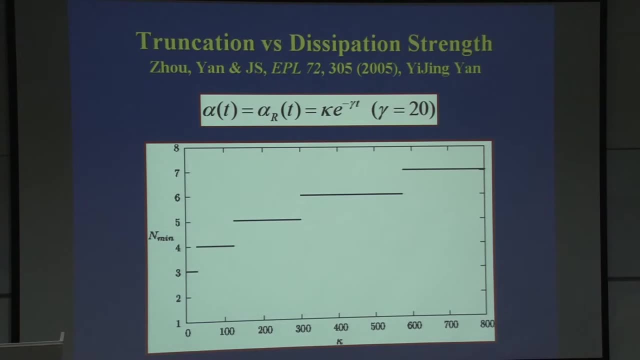 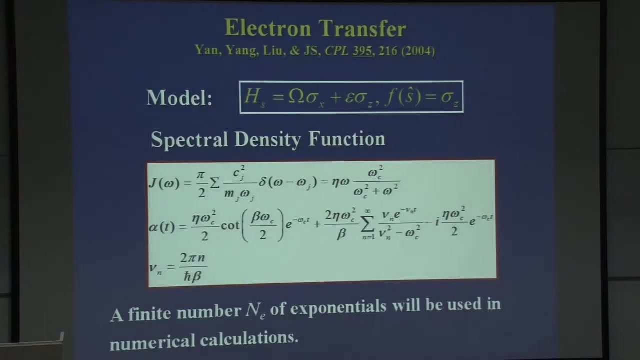 This is why it works, at least from our theory. You can understand this very simply. Now we test the deficiency with respect to the dissipation strength and the memory length, And I will skip this and also this one And we'd like to talk about. 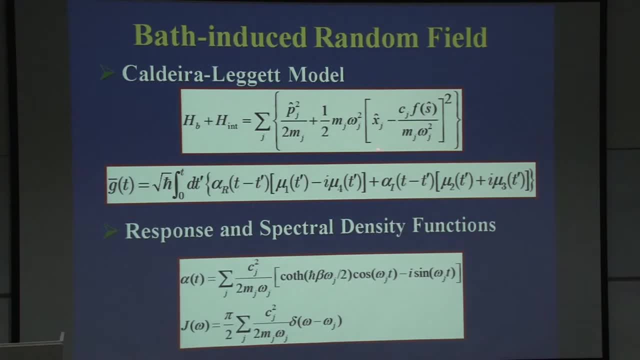 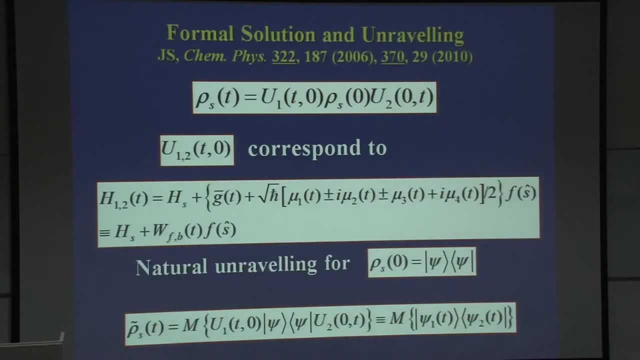 more realistic model, the counter-length model. It consists of the bus, the harmonic monitor bus, because again it's linear. You can write down the bus-induced field, blah, blah, blah, And we also do some analytical analysis deriving the mass equations. 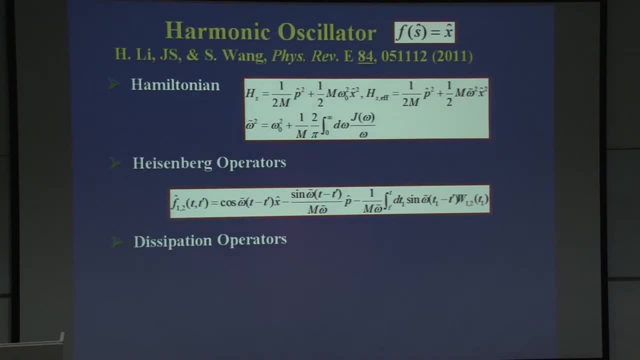 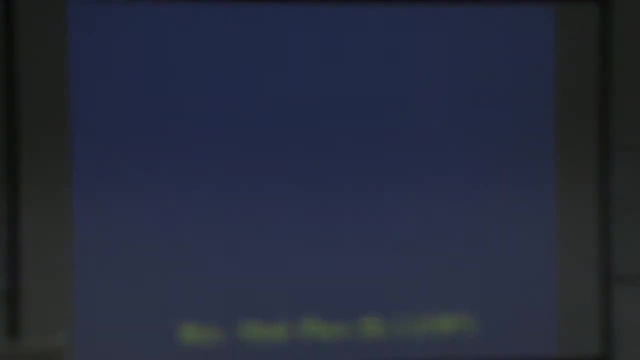 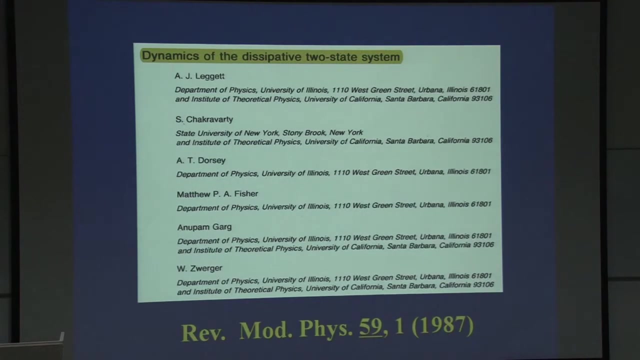 for linear systems, I will skip all of them And to look at the really challenging problem of this Bing-Watson model here, this very influential paper published in 1987, Dynamics of Dissipative Two-State System. very simple one. 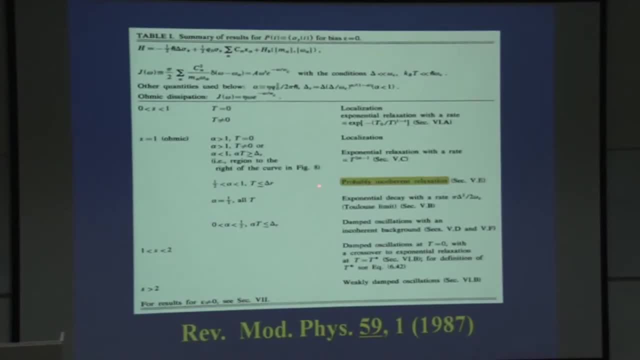 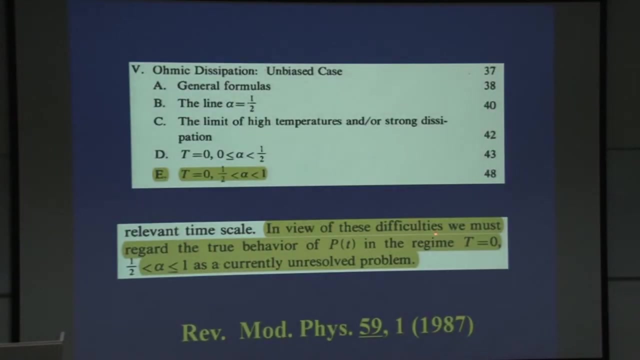 And there is a table that tells us that when temperature is very low, there is a range that the dynamics is unsolved up to now, still every 10 years. So, in view of these difficulties, we must regard the true behavior of this population, of the two-level system. 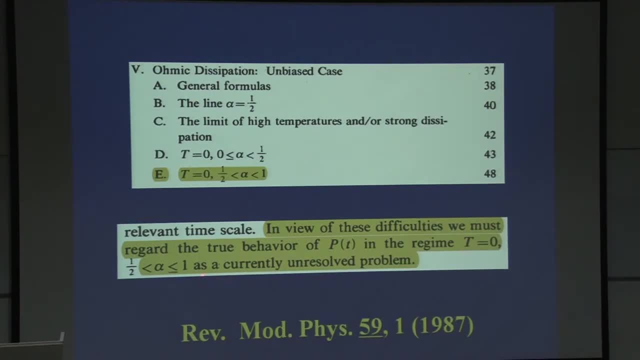 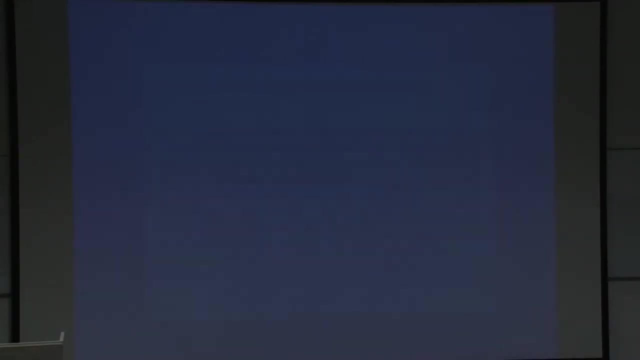 the dynamics at zero temperature for this dissipative strength is unsolved. This is why we developed our methodology in order to answer this question. In Westbrook also, there is a similar statement for our Bing-Watson model, where we have a very, very 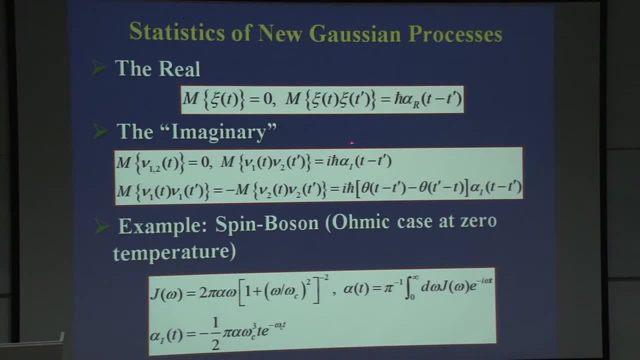 challenging problem. Now we can combine the wet noise and the bus-induced field in order to enhance the sampling efficiency. So for the Bing-Watson model. again, the question is: the noise is long-ranged in time, Of course. 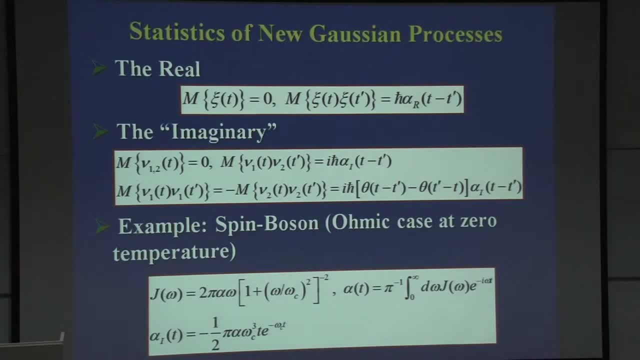 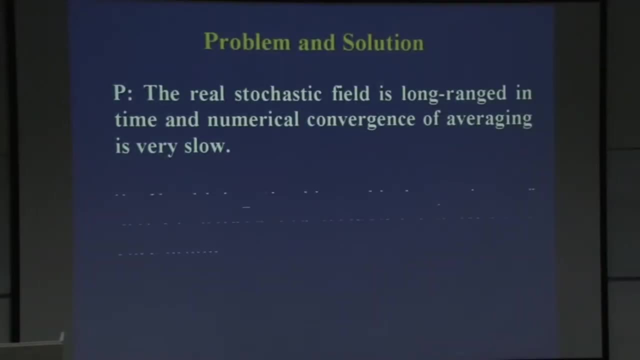 the hierarchical equation of motion works. It works only for exponential decay, So it doesn't work at zero temperature, as Yijing has already said. Now, in this case, how can we do? One way we think out is that we combine the hierarchical 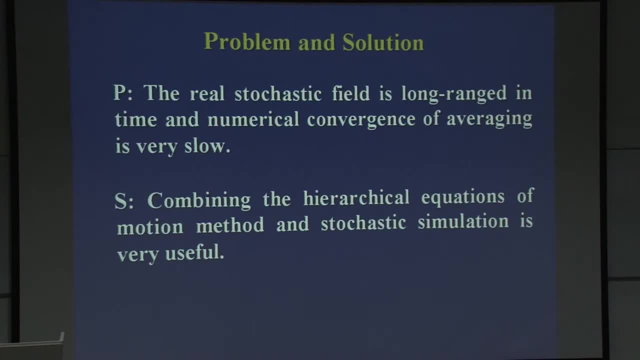 equation of motion method. It is deterministic, it is effective, but it's specific. With the stochastic simulation it is very general, but the efficiency is not that high. So we have to take both advantages of the two approaches so that we can do something. 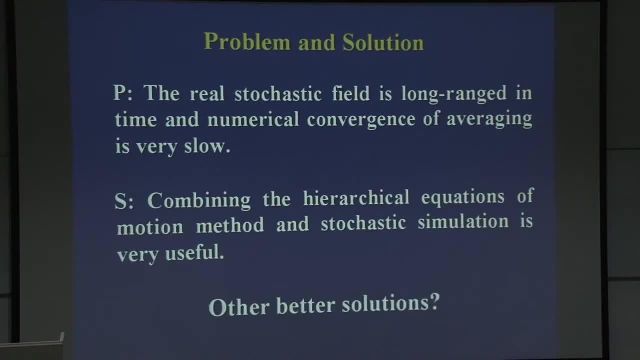 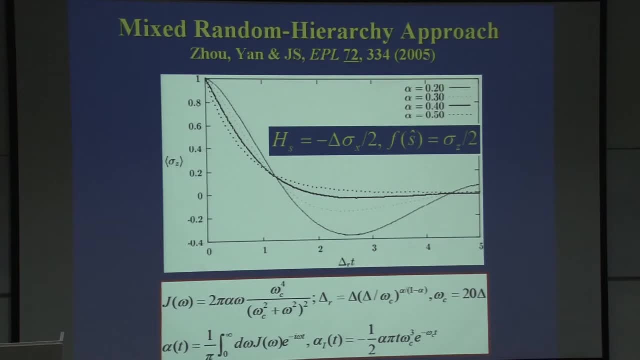 This is our idea to tackle this problem. OK, Let's show you the simulation we've done. Again. alpha represents the dissipation strength. If it's smaller than 0.5, it is similar to underdamped harmonic oscillator. this quantum coherence. 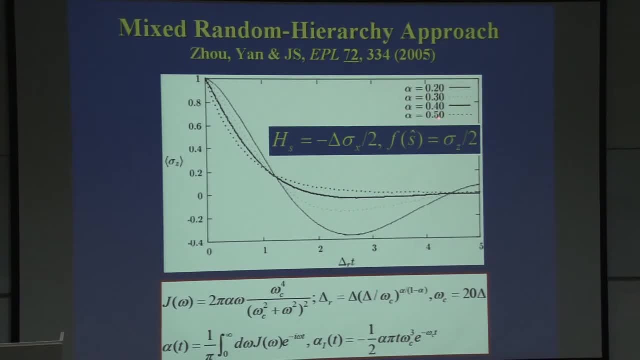 you will see from the dynamics of the population And the transition between 0.5 and 0.5 is the same as the transition between 0.5 and 0.5. So you can see the difference between 0.5. 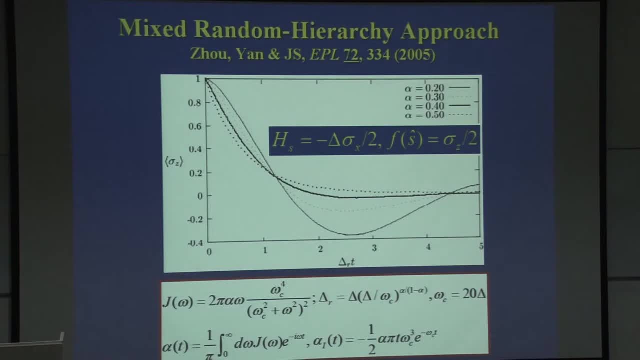 and 0.5 and 0.5.. The transition from coherent to incoherent, to motion, is at this specific point. It's called solid-solid limit. Actually, the spin-boss model for this parameter can be transformed into a solvable model. 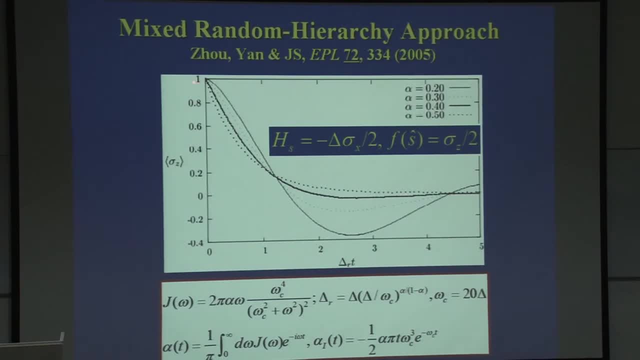 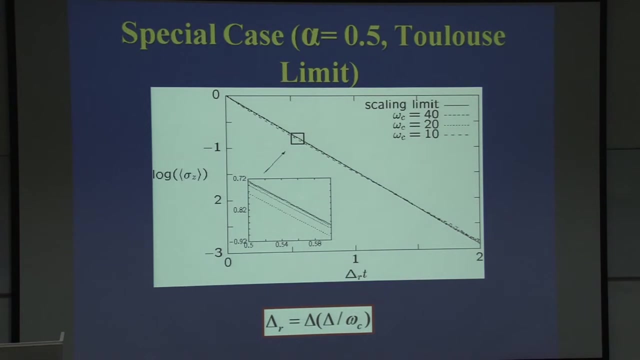 So you know the effect dynamics. We do the simulation. The result is consistent with previous theoretical model of prediction. Well, how about strong dissipation? This is really a problem we try to solve Increasing the dissipation strength. we find that 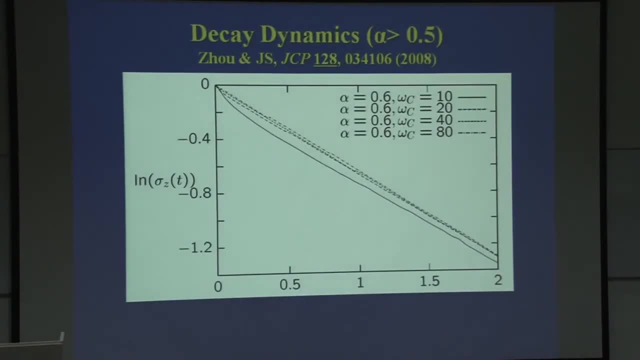 OK, again, the dynamics is rather simple. It's exponential decay. This is for 0.6.. The puzzle we have had is the following: Now the time scale again. perhaps I should explain a little bit about the time scale. 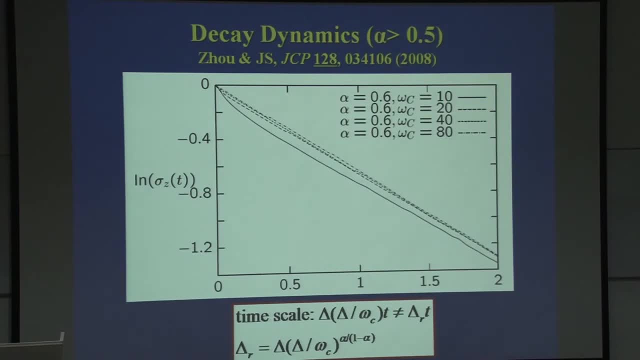 For a barrier two-level system. the time scale is dependent on the intrinsic frequency. It is dependent on the undisciplining, But when there is an environment, frequency is modified. according to some law, It can be resolved by using renormalization. 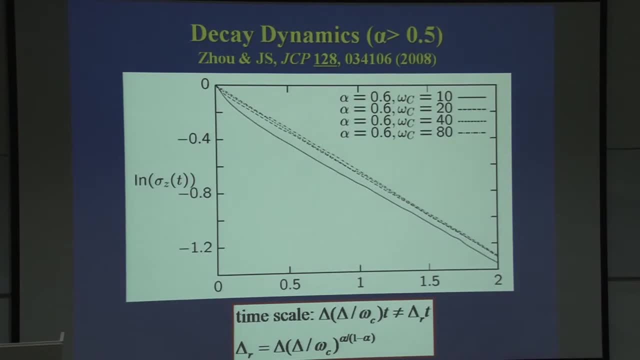 theory. It's simple, But it only works when the dissipation is weak. So we really find that when dissipation is weak, our simulation is consistent with theoretical. I mean theoretical simulations Okay, but for the stronger dissipation. 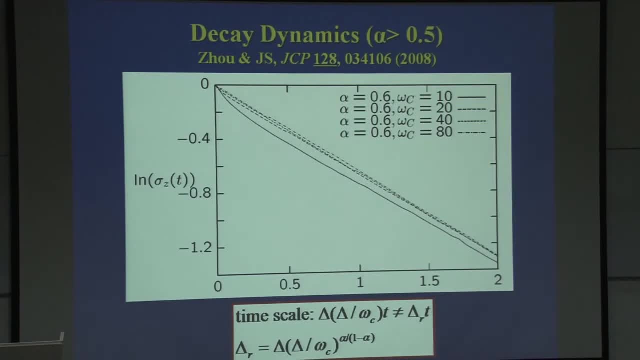 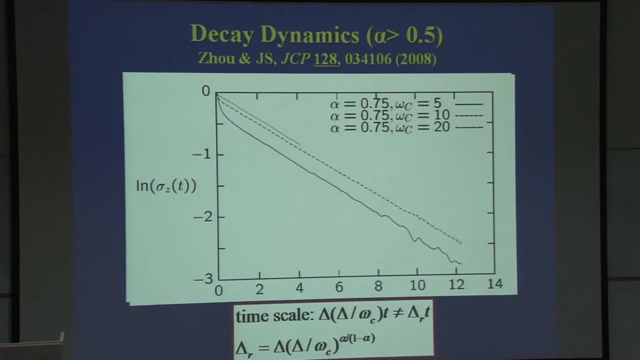 we found that the time scale will not change after the coherent and incoherent transition. We don't know yet what the physical mechanism and or the underlying physical principle. Now we do quite a lot by increasing the dissipation strength and also the high 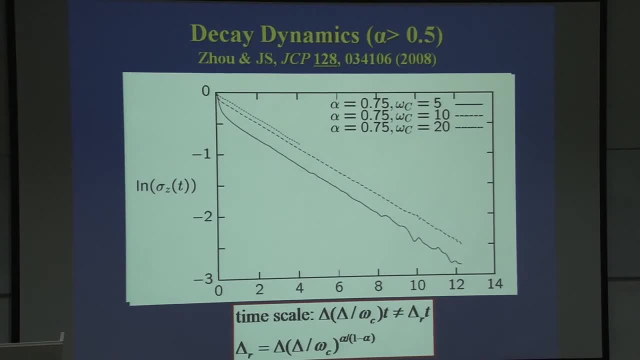 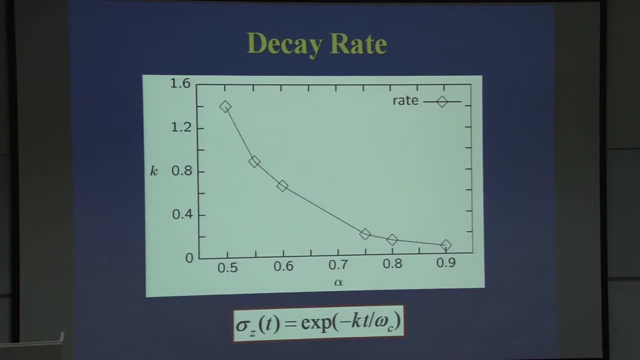 frequency cut-off. I mean not to get into the details, but we'd like to use this very simple graph to tell you what we have done. Okay, At this point, we know that other theory is exponential decay. We have shown that. 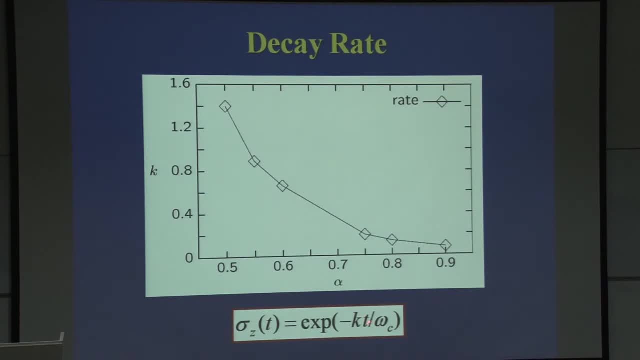 the decay rate is modified by a factor which is 1 over the hair energy cut-off, So increasing the dissipation strength. we have smaller rate constant. The decay rate is smaller and smaller When the dissipation strength is 1, we have 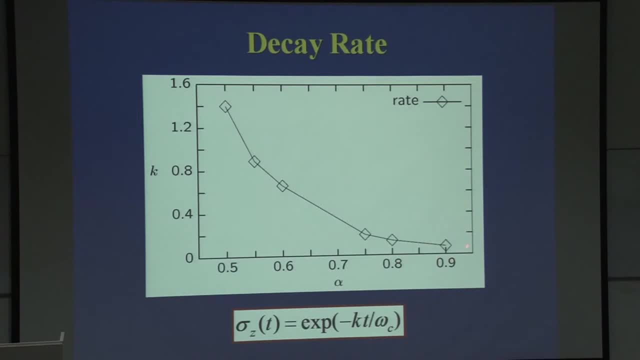 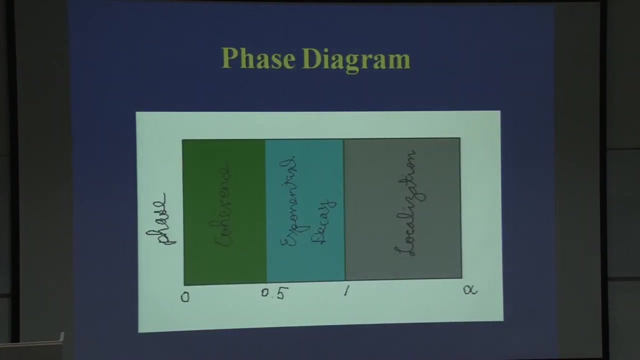 quantum phase transition, But our numerical methodology does not allow us to reach that form. We stop almost here, So there's still a gap. Now let me use this index of the dissipative two-level system. If the dissipation strength is: 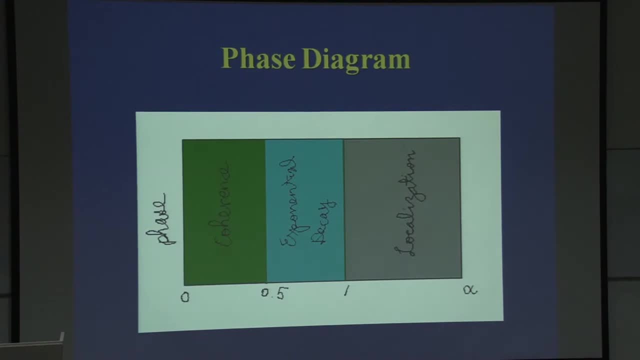 not large. then we have quantum coherence. Many people in quantum information will be happy about that. It's no problem. Well, when the dissipation strength is 1, we are happy with stable configuration. But in this range, this unexplored- 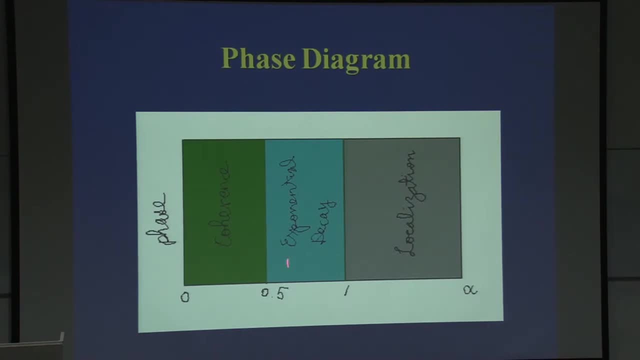 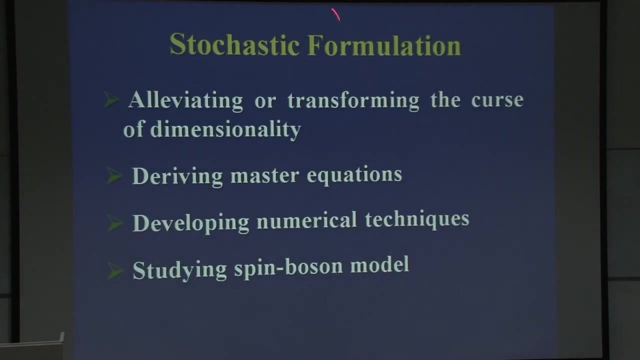 region which is corresponding to quantum physics. But again, we have worked out some results from the whole. But to summarize what we have done, we tried to set up a stochastic formulation so that we reduce the number of dimensions, so that we can use it. 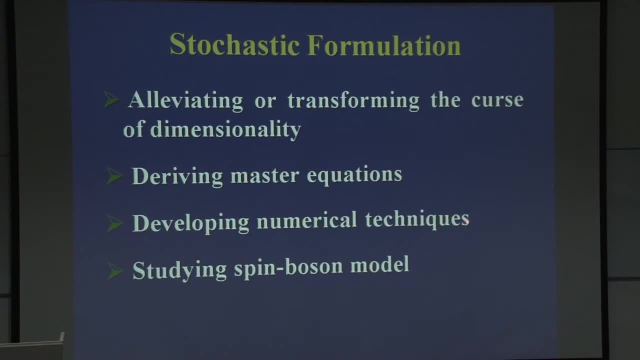 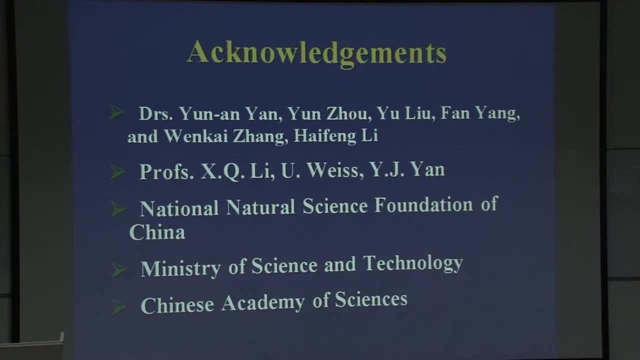 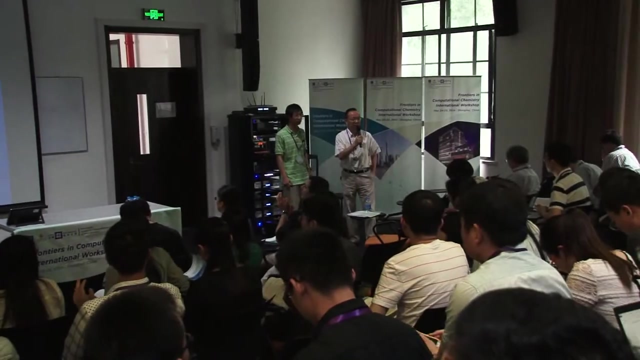 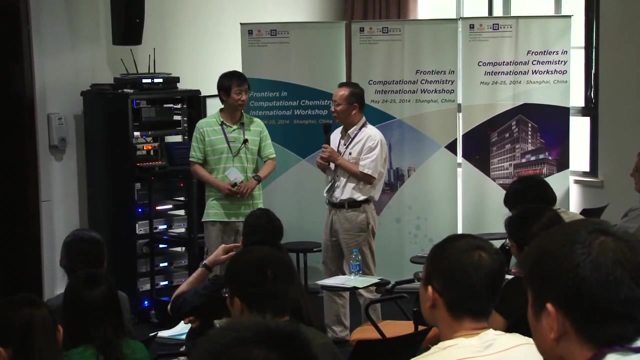 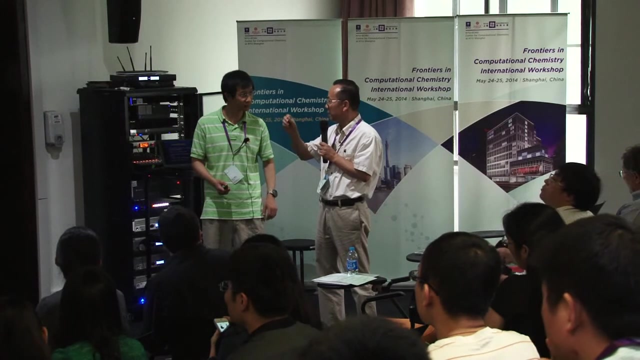 either by equation for linear systems or to do some real simulation to solve a problem, And we have a lot of data available to my co-workers and friends and the following agencies for continuous support. Thank you very much for attending. So any questions? So? 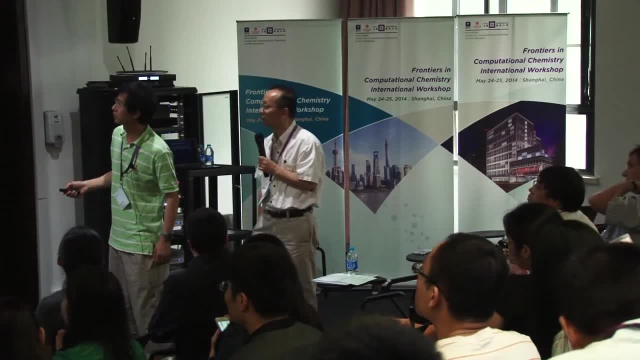 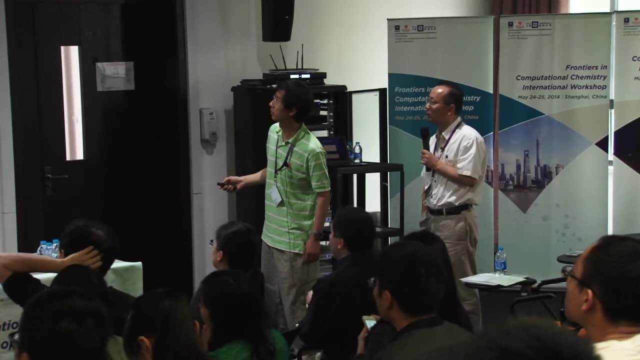 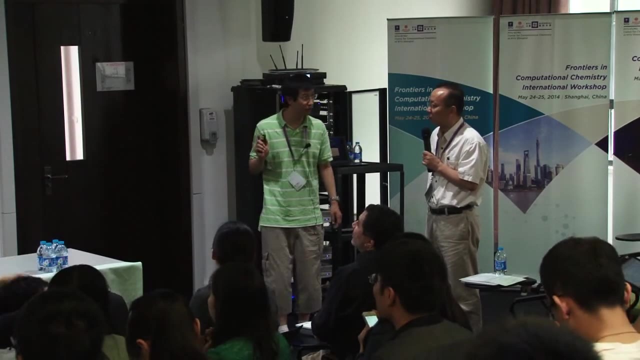 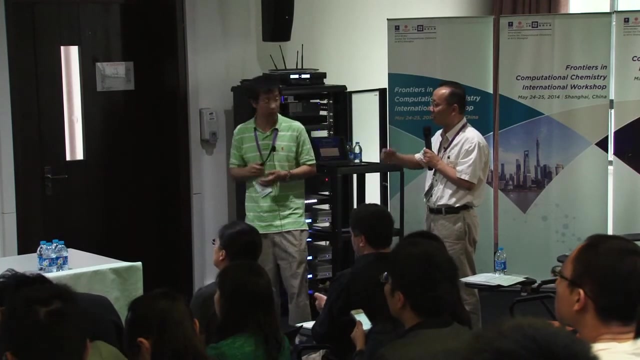 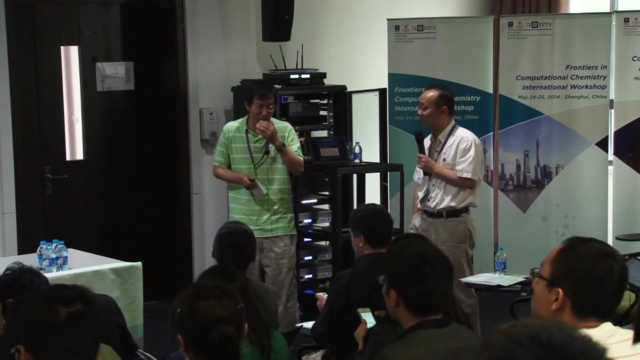 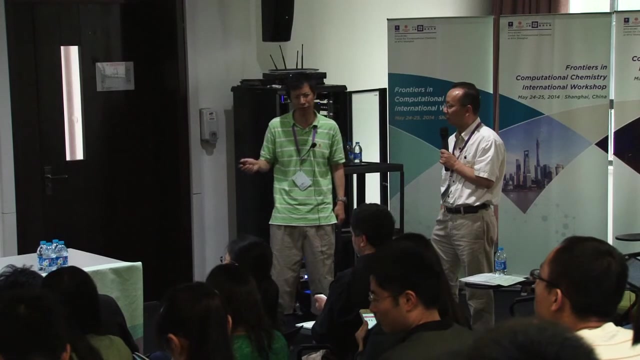 I would like to ask a few questions from the audience. So I would like to ask a few questions from the audience. So I would like to ask a few questions from the audience. You can directly relate it to: the well have to parameterize so that.